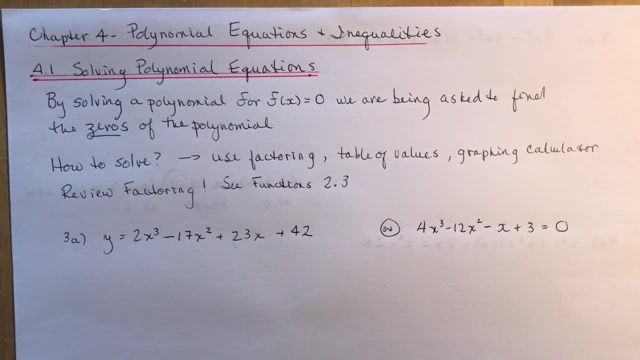 spectacularly new for you in your understanding of solving equations, because you've solved a lot of quadratic equations, So now all we're doing is looking at equations that have higher degrees, and because we've already done some work in the previous chapter on how to factor cubic and quartic functions using the factor theorem and the 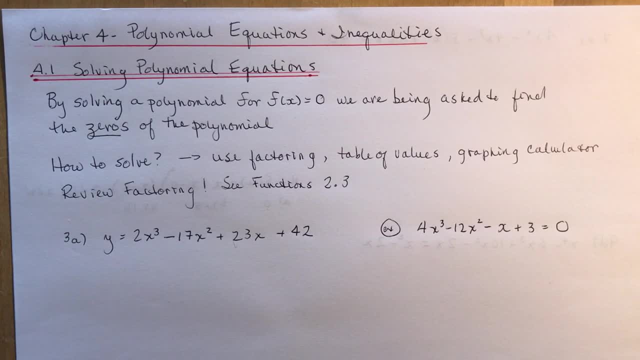 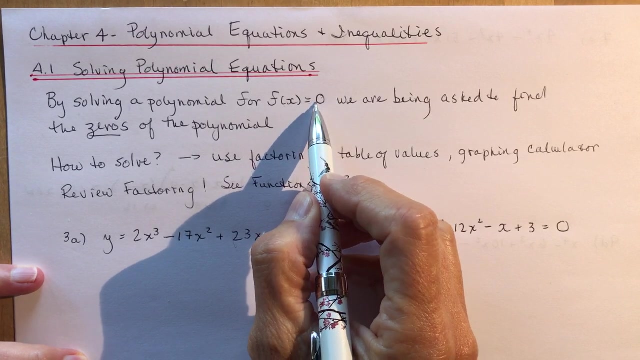 remainder theorem. you should be pretty good at doing this by now using synthetic or long division. So when we solve a polynomial function, we're solving it when f at x is equal to zero, and what this means is that if your equation is not set equal to zero, then you need to move everything. 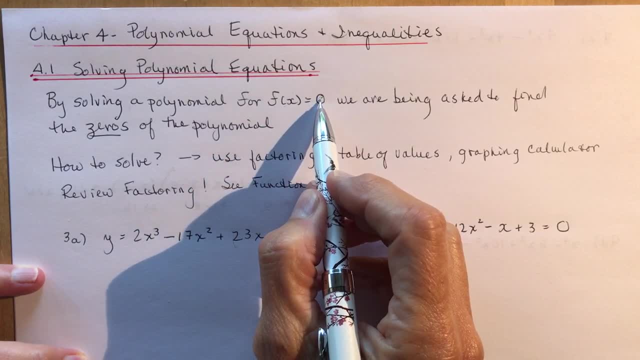 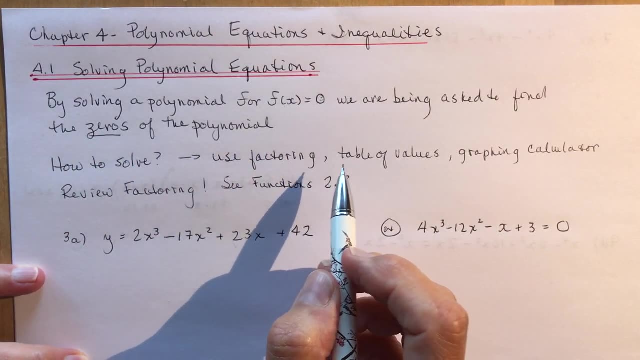 to one side of the equation so that you can have a polynomial equation. So if you have a polynomial, you have this little happy zero face and then you will be finding the zeros of the polynomial. So that's really the important thing to remember to do, because sometimes people see equations and they 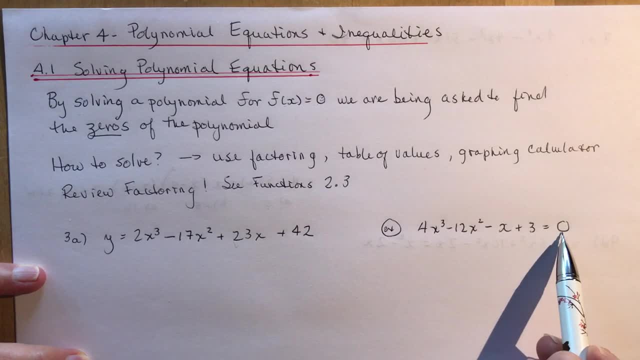 go. oh, what am I supposed to do with this? and when you see it set like this equation over here, you would know right away that this is set to zero. You're solving what makes what value of x put into this equation will give me zero for an answer, and of course, those are the zeros of your function. 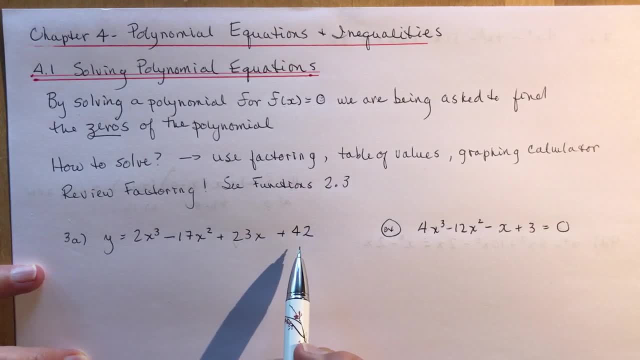 So let's take a look at 3a here now. in this part we're just solving equations, not inequalities. that's the next little thing we're going to look at, and the first thing you're doing here is you're trying to solve this equation. So I want to set this equation and I'll write it out again, just. 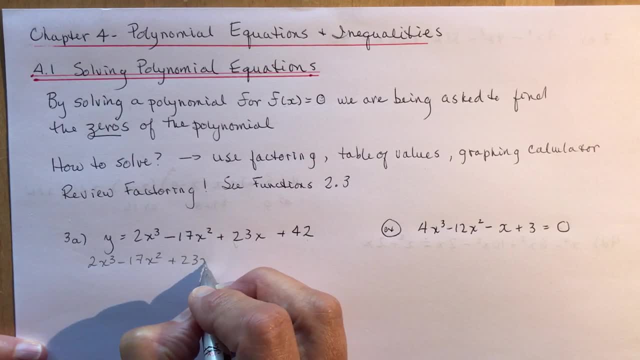 so that it makes me more comfortable knowing that it's not y. but oops, pushing too hard, so excited to get going on this lesson, so I've set it equal to zero, and if you recall from the previous lesson, you need to find the factors of 42 and something needs to make this equal to zero. now, the sad story is that not. 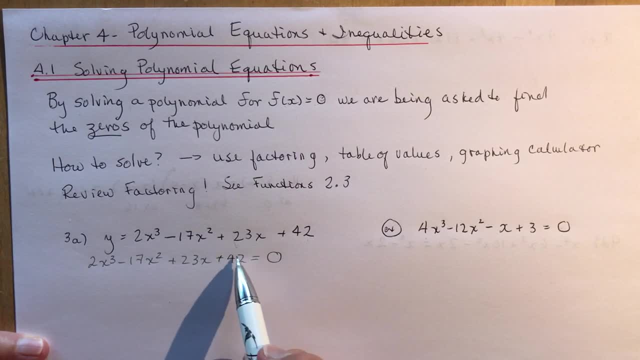 everything is factorable. so you might go through all the factors- not in this case. but you might go through all the factors- only to find out that nothing makes this equal to zero, in which case you're going to be very sad. so let's say we'll do f at 1 and see what happens. so we put in 1. 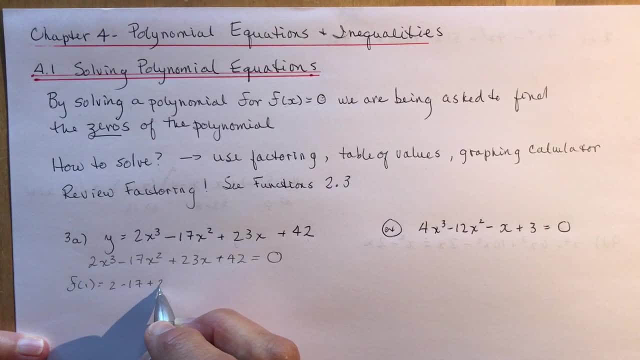 and we would get 2 minus 17 plus 23 plus 42, that's f at 1. this function at the value for 1 and you can see that that's 44 minus 23 and 1 is 4 um 30. I don't sorry, what am I doing here? 45, and it's not zero anyway. so f at 1 is not equal to zero. 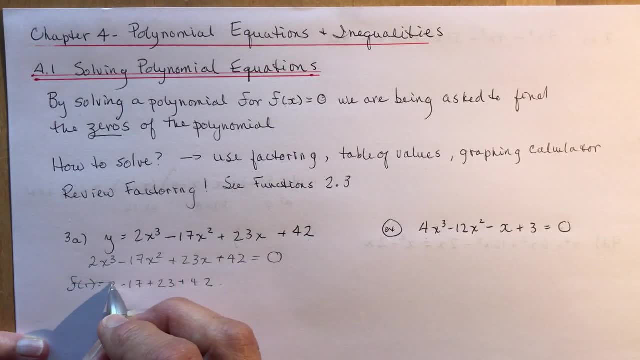 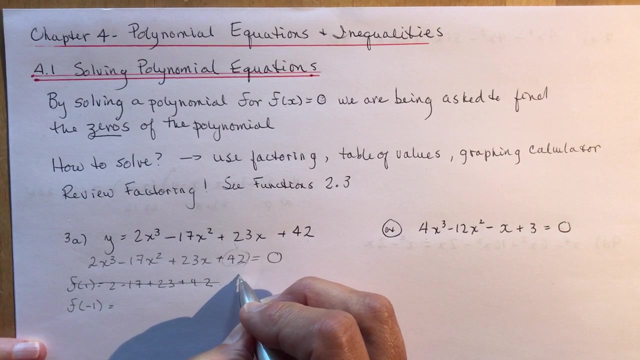 so let's like scratch that one off your list. so then you might want to try f at minus 1. there's no point in going to really high numbers now. you know all the factors of 42, so you would have 1, 2, 3, 6, 7. 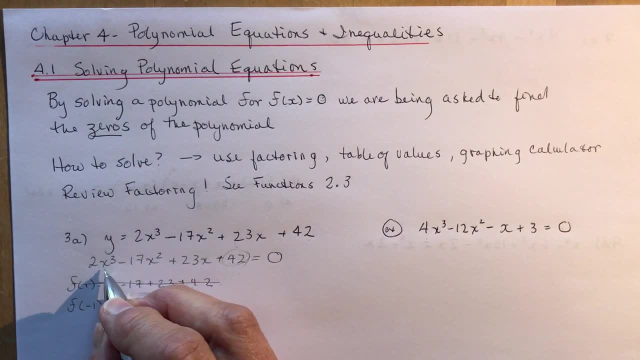 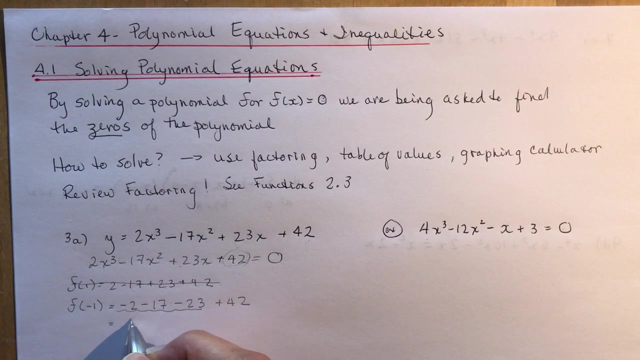 and the plus and minuses of those. so I'm going to try minus 1 here. so minus 1 here is going to give me minus 2, minus 17, and then minus 1 is minus 23 and plus 42, and you should be able to see that this, all these negative ones here, are negative 42 plus 42. 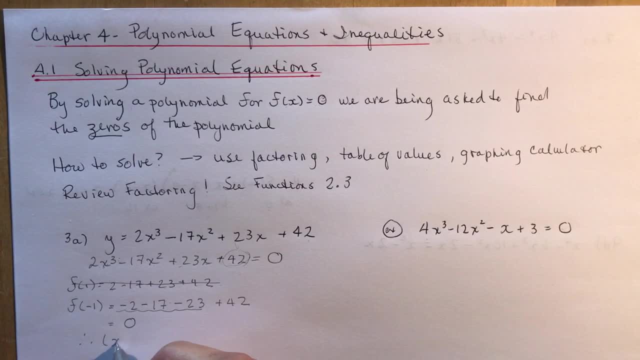 is zero, so that means that x plus 1 is a factor of 42. but you still had to work this log out, I name it that you go in the show a little bit of room when everybody was calling you here and you had to seem to your perspectiviall. nesse doesn't mean f, ㅎㅎ that. but yeah, you could find this at ff at 2.60.1 of a home dollar for yourself. let you, if there's Anastacia going. 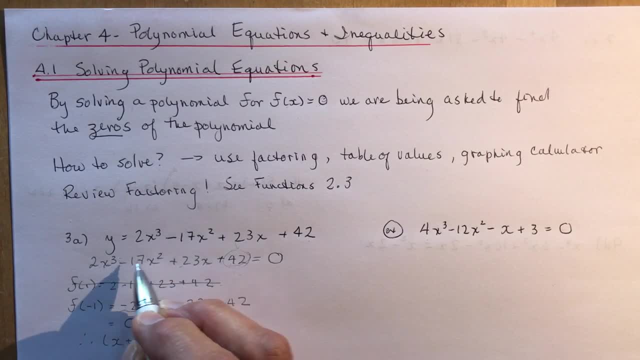 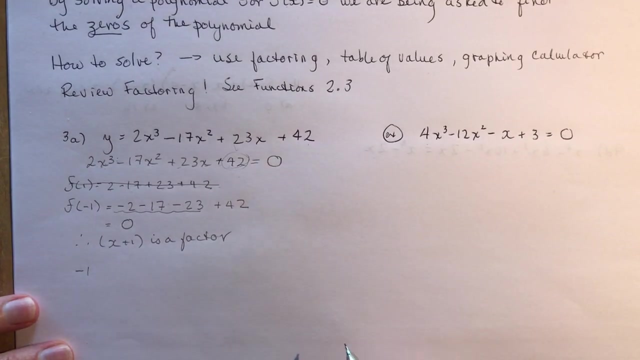 it's a factor of this polynomial. and when, when this function, when x is equal to negative one, that would be one of the roots. so when i do my synthetic division, remember you use the root. if i'm running out of the paper here for you, so you put the minus one there, you make your upside. 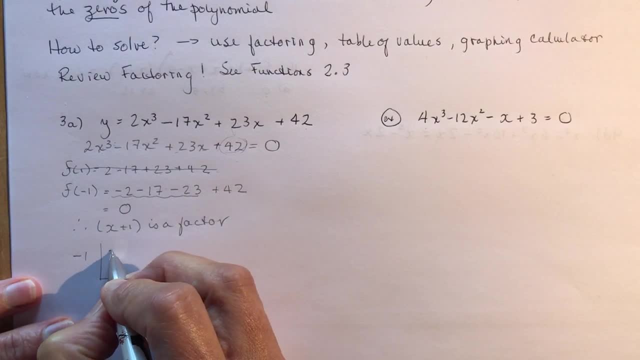 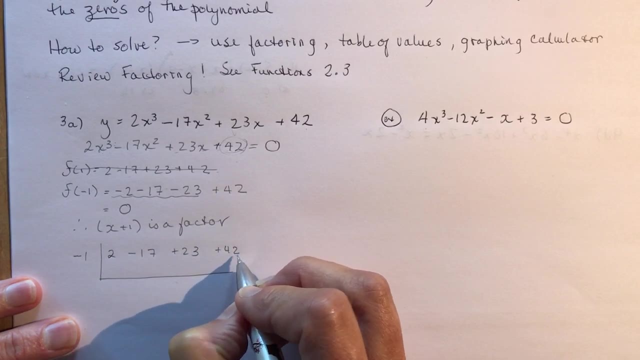 down division sign and you put in all the numbers. so i have 2 minus 17, plus 23 and plus 42. i bring down the first number, which is 2. i multiply it by minus 1. i add these together. multiply by minus 1, this times minus 1. i add them together. i multiply this by minus 1 and i get 0. 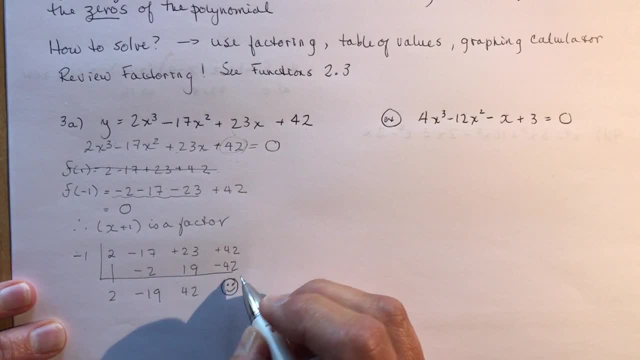 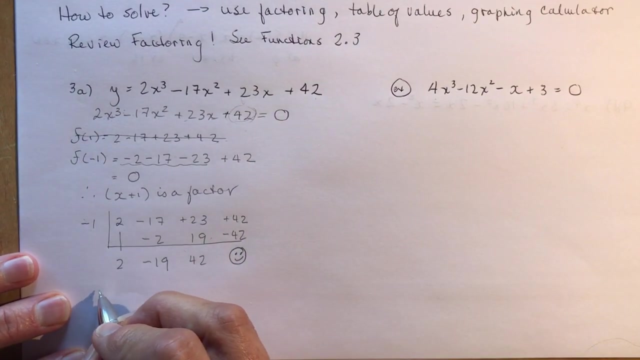 now you know that if you don't get a 0 here, then either you made a mistake in the calculation here or here, and then you go back and fix it, okay. so i know that minus 1 is a factor, or, sorry, x plus 1 is a factor, minus 1 is a 0. and now i know that. 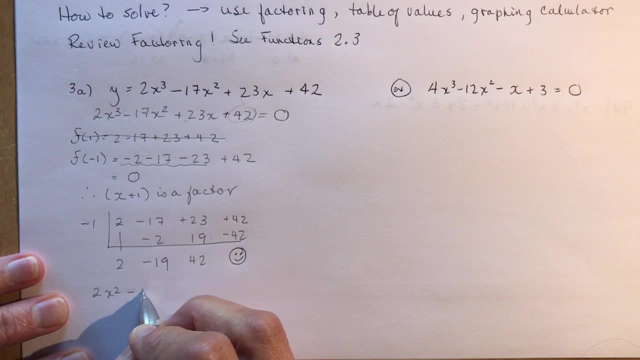 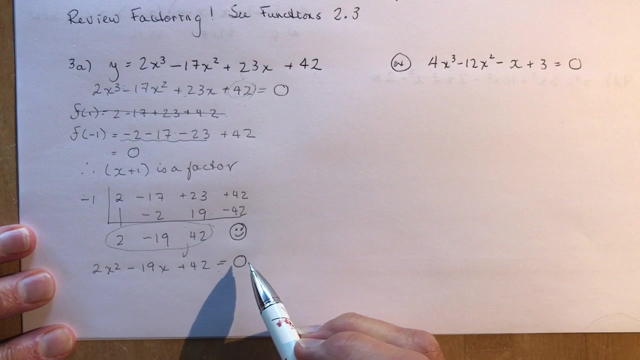 what i have left here is: i have 2 x squared minus 19 x plus 42 is equal to 0, so that's what this gives me right. so now i need to factor this. now, if you have a, if you have trouble with factoring, you should go back and take a look at some of the practice. 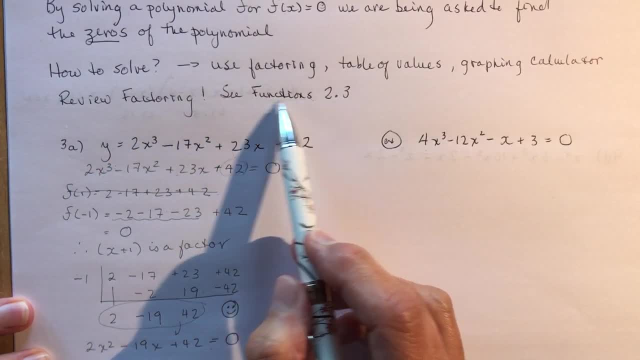 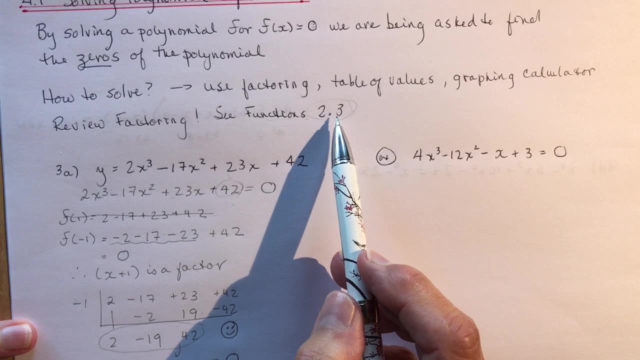 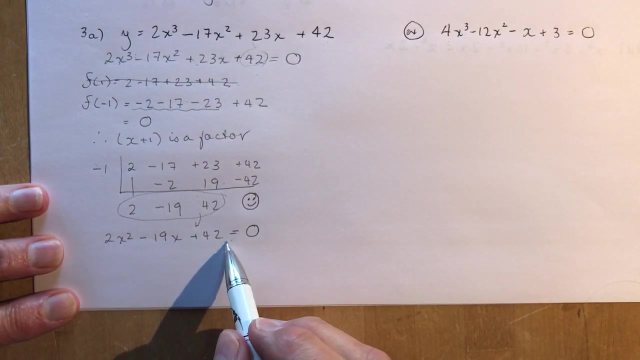 in functions 11- so that's my first set of lessons that i did- and 2.3. there's three or four different videos talking about the different types of factoring. if you need to review that, okay, so let's go down here and again. we're going to factor this, so we're looking for a product of. 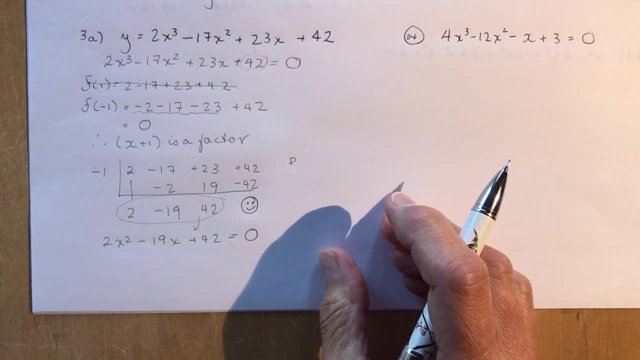 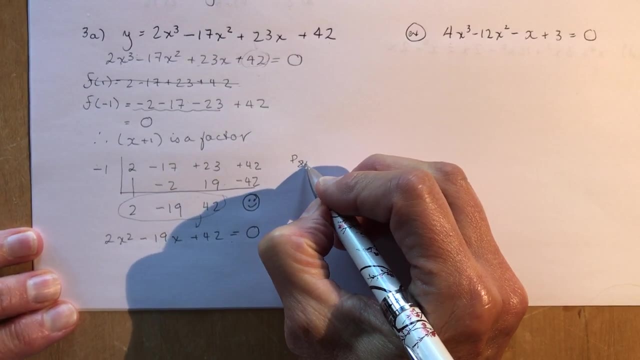 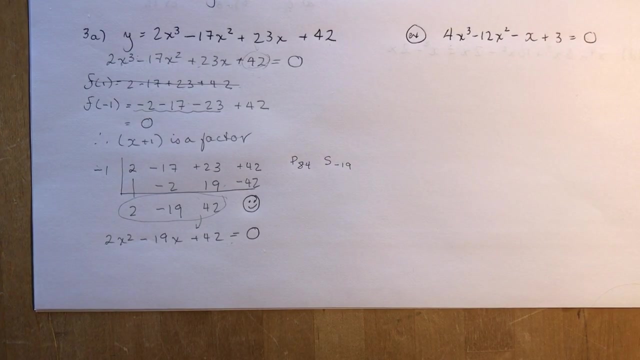 the first and the last. so the first and the last here would be 84.. let me see if i can add another little more light here. so product of 84 and i have a sum of minus 19.. so now think about all the numbers that multiply to. 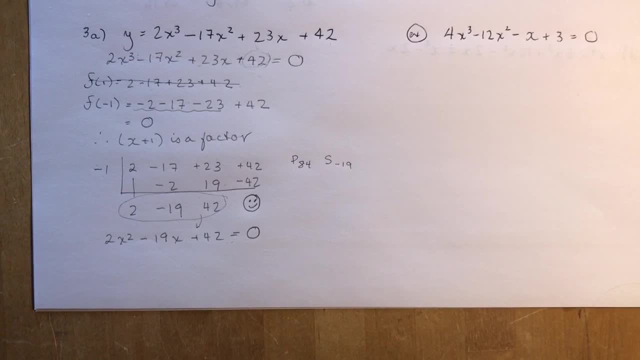 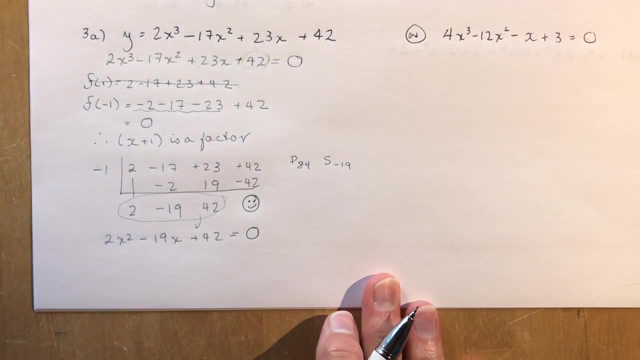 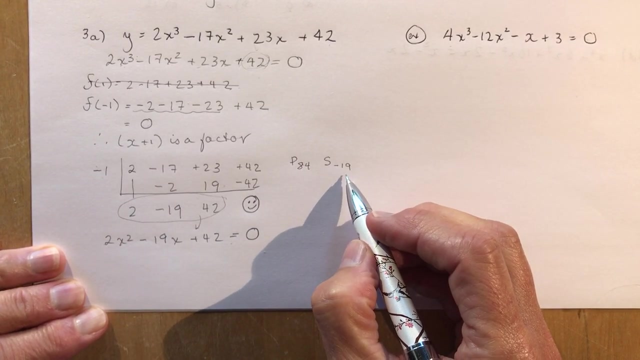 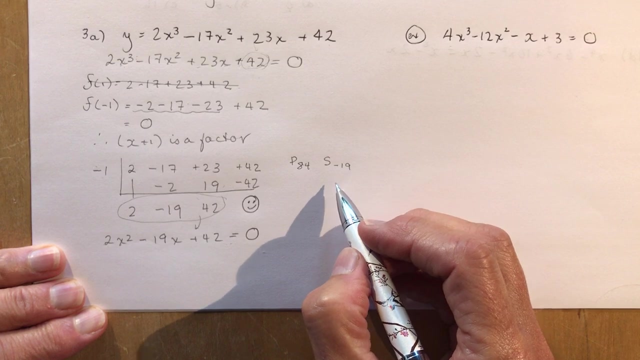 to 84 and add to 19.. let me try this. this help there. we go a little more light here, okay, so, product of 84 sum of 19. how about let's see 19 minus 19, sum of minus 19 and a product of 84. so. 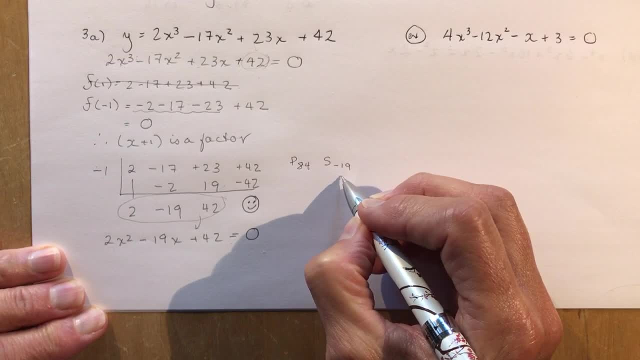 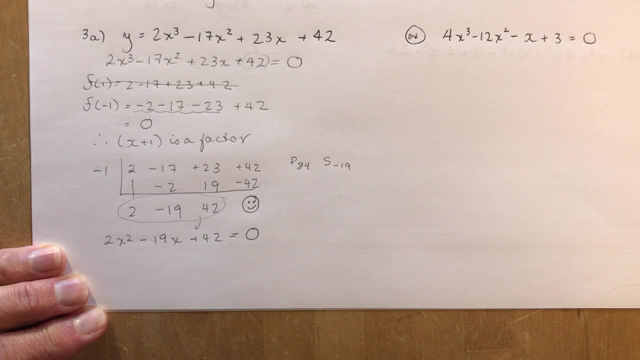 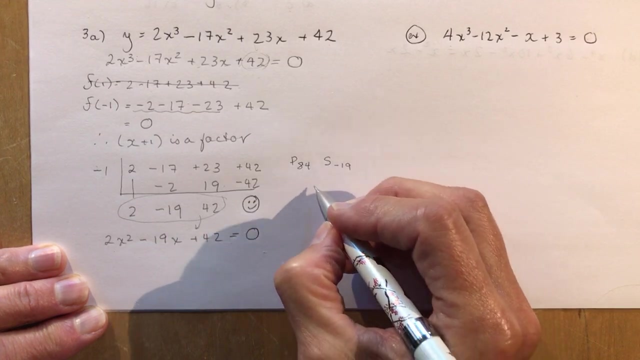 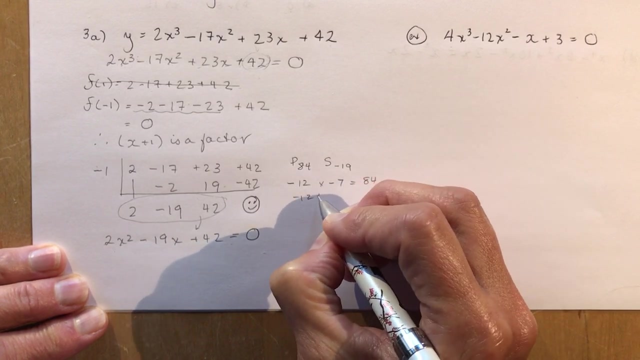 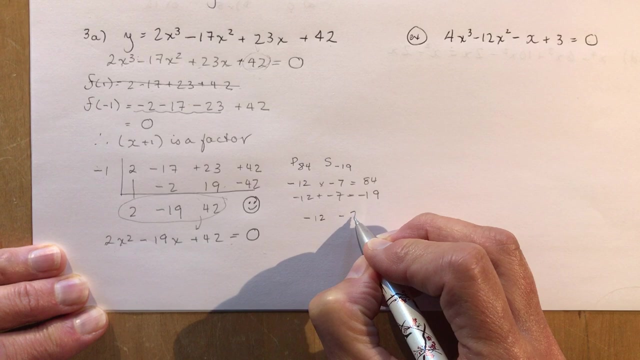 what works, guys, help me out, help me, branda, i know what's doable. 12 and 7, right, okay? minus 12 times minus 7 would give me 84, and minus 12 plus minus 7 would give me negative 19.. so those are my two magic numbers. i write them out again and the easiest way to factor. 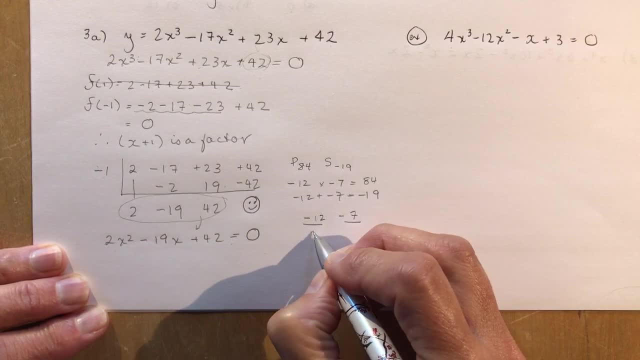 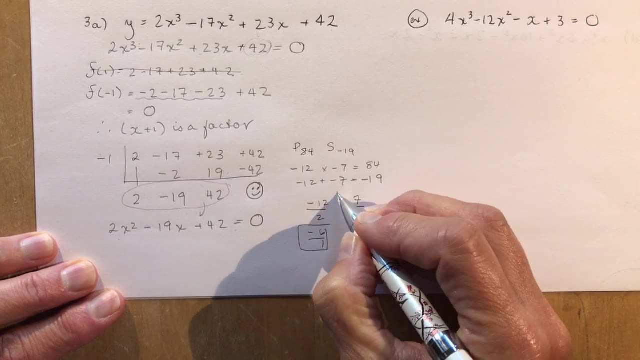 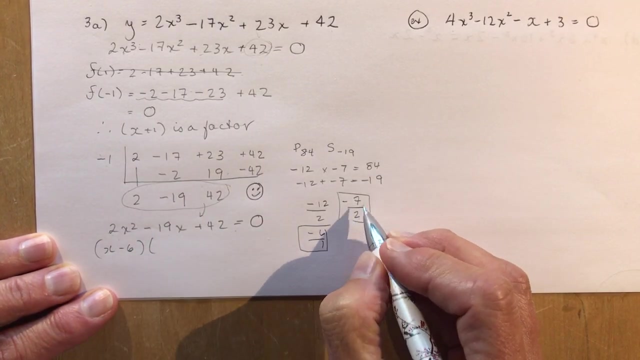 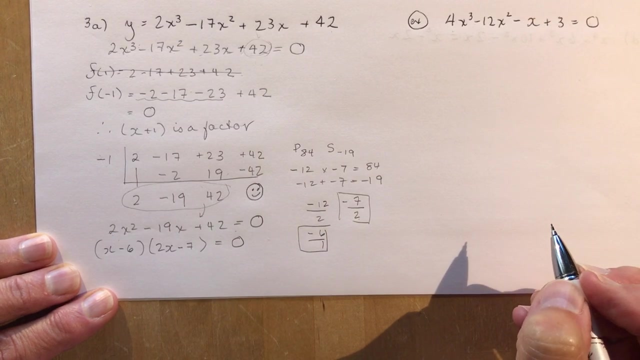 now is to put the coefficient of x squared underneath each and reduce your fractions. so that's going to give me minus 6 over 1 and this one is done. so this factor is to be x minus 6 times 2x minus 7, and my other factor: well, that's just that one, okay. so if they asked you just to solve it, you'd say: 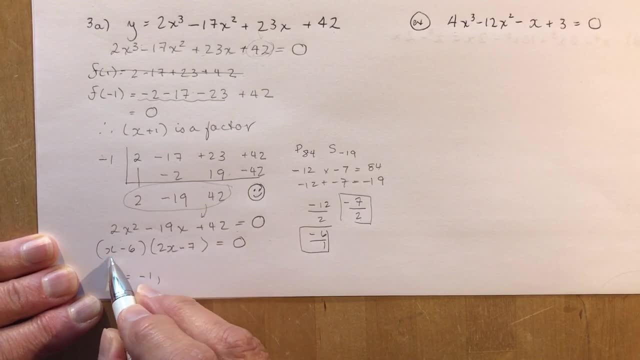 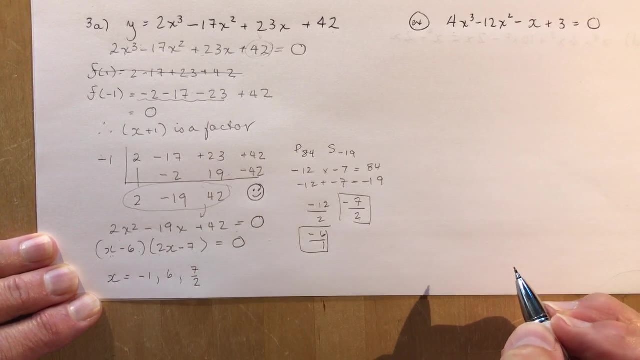 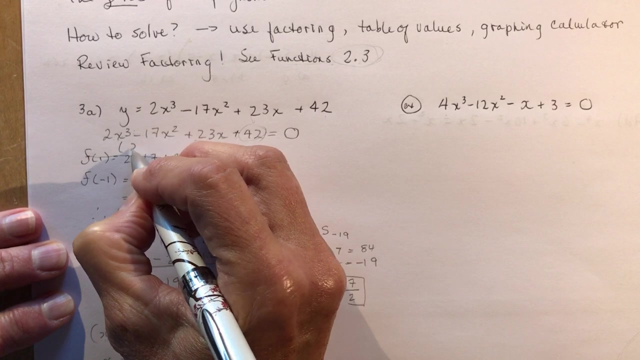 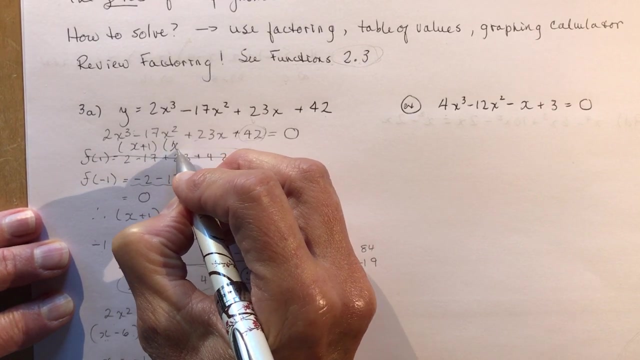 well, that means that x is equal to negative one. what makes this bracket zero? you would say six. what makes this bracket zero? and that would be seven halves. so that means that this equation right up here, this is the same thing as x minus x plus one, sorry, x plus one times x minus six times two, x minus seven. 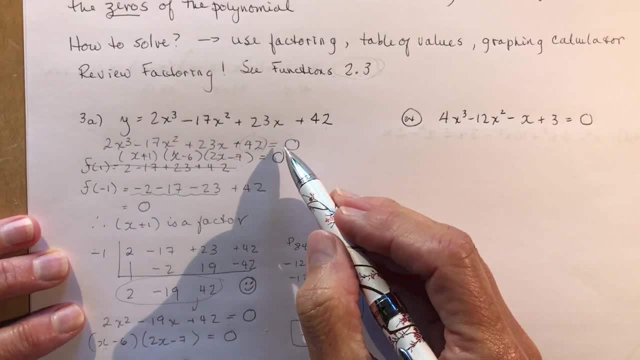 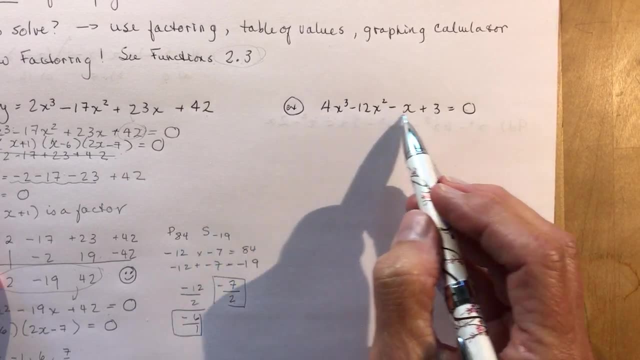 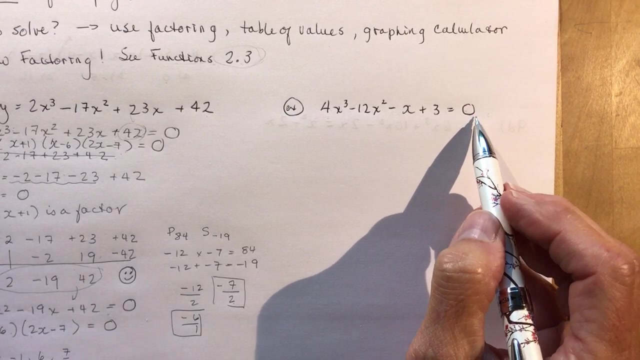 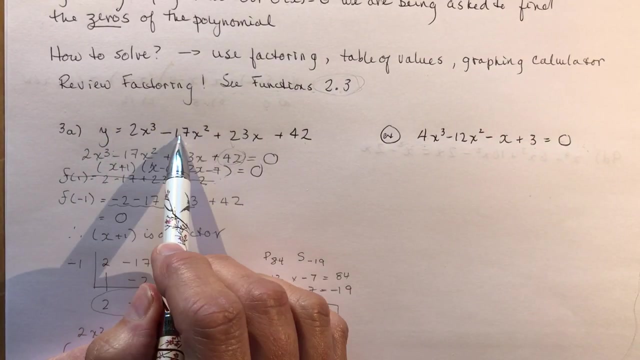 that's another way of writing the fact, writing out this equation, writing it in factored form. okay, so another thing you might have to factor would be something like this: it's another cubic function. now, what you should always look for first is to see whether or not this can be factored by grouping. now, this one, you can see there's, there's no. 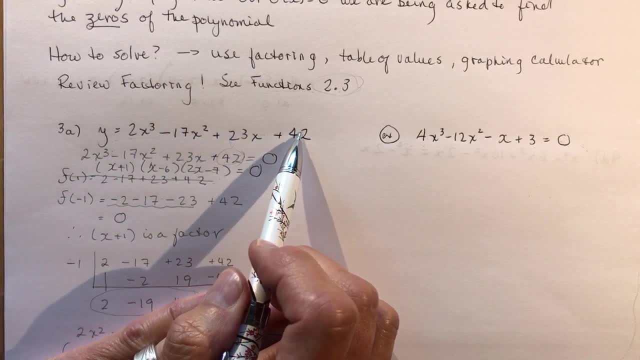 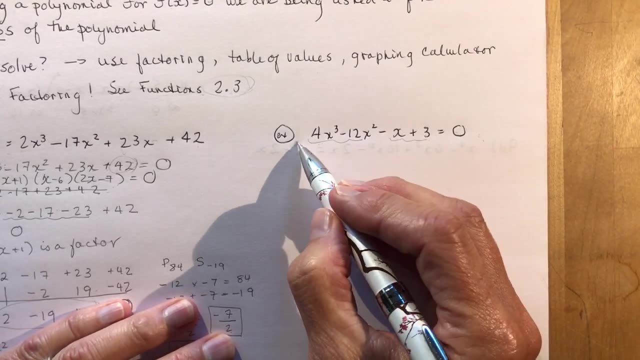 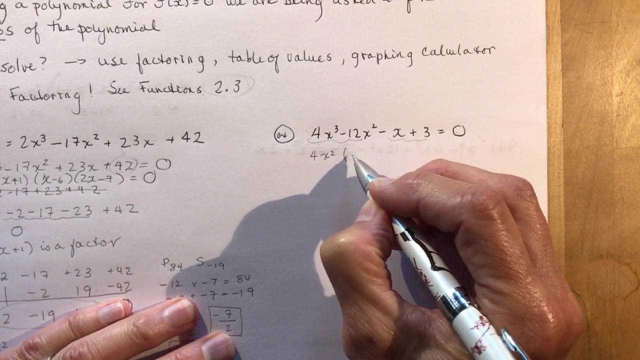 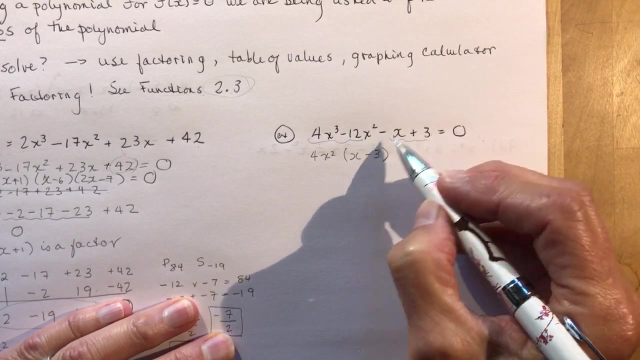 factors. no way you could factor this as a group, but this one, if you look at these two and these two and you pull out a common factor here. so that would be what we could take out: a 4x squared right, 4x squared and i'm left with an x minus three, and this looks kind of like that. 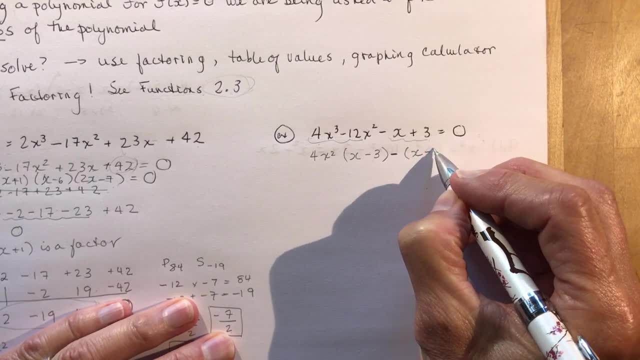 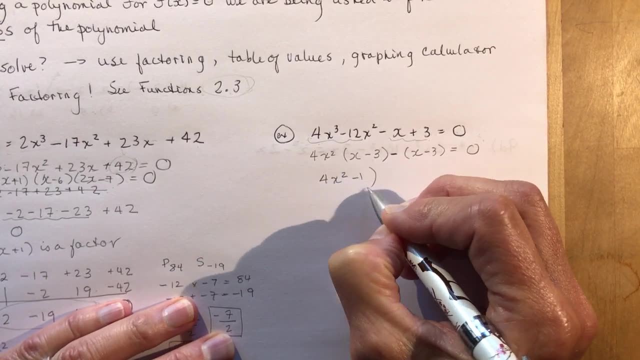 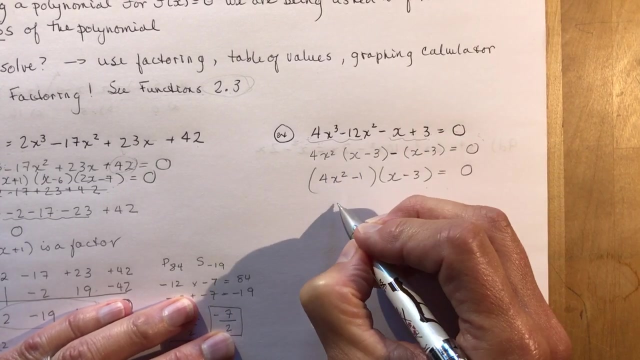 but it will if i take out a negative one. so that's just to make sure that you don't waste a lot of time trying to factor these things when it's just as simple as doing that. okay, so if i wanted to solve that, i would say x minus three and i would take out a negative one, and then i would take out a. 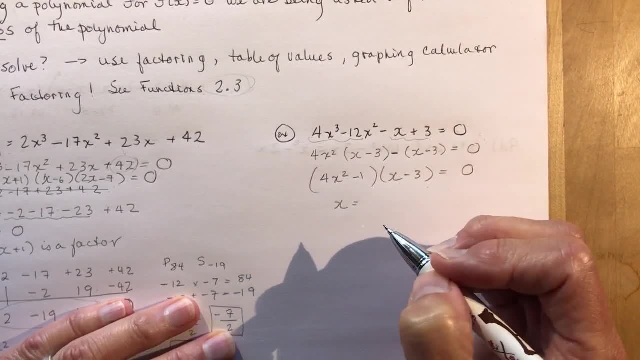 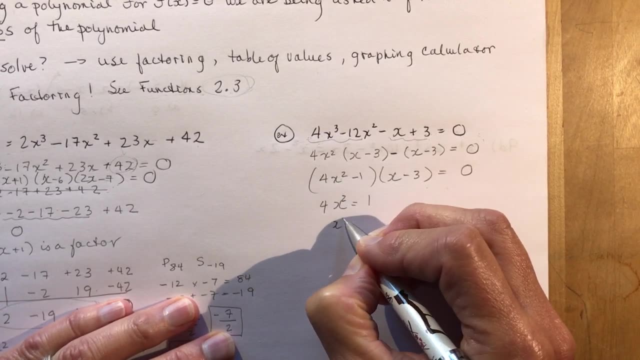 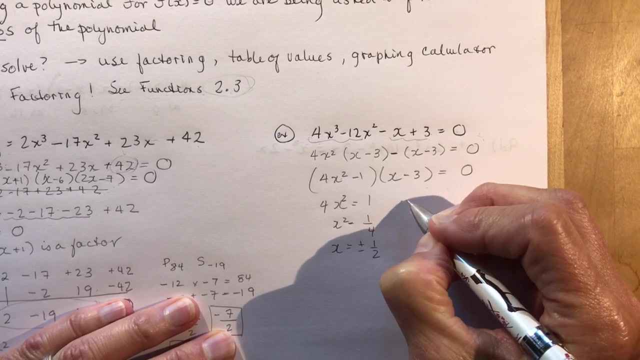 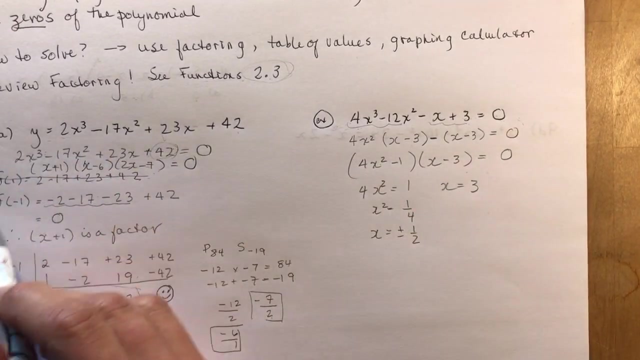 x is equal to- um, sorry, i would have had 4x. squared is equal to. 4x squared is equal to 1. x squared is equal to one quarter. so x is equal to plus or minus one half, and this one would be. x is equal to three. okay, so don't make your life difficult by doing a long factoring like this when. 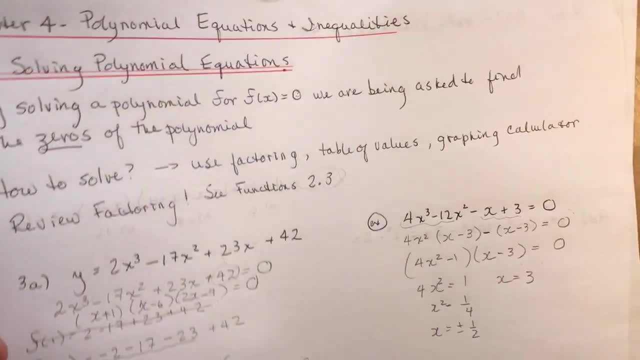 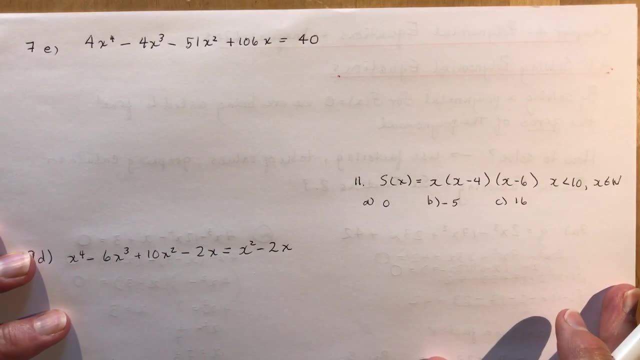 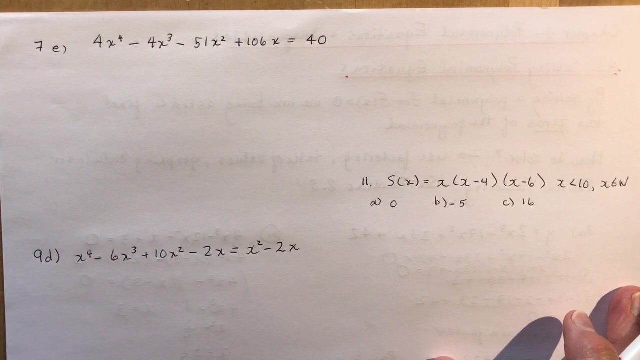 it could be factored by grouping, so always check. okay, let's move over to another question. these are questions from the homework, because the textbook- um, i think it's very wise if you read the examples in the textbook rather than me just writing them down here for you. so this time, 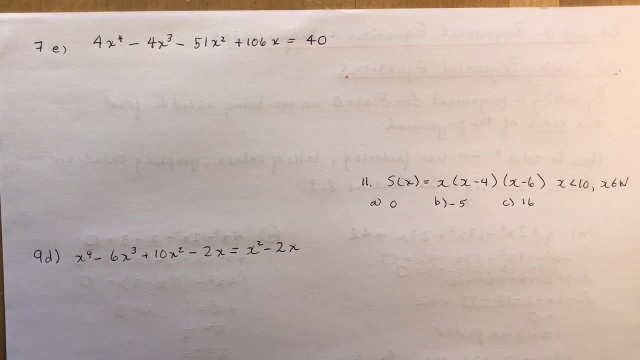 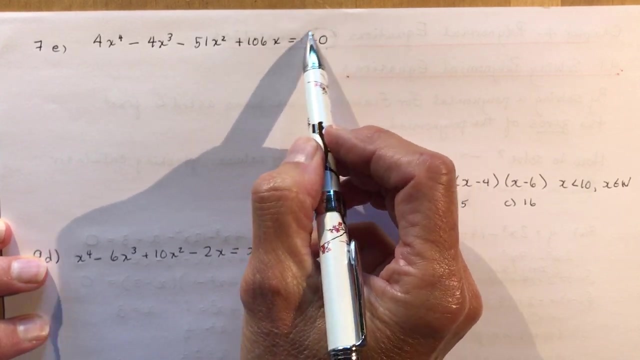 i chose to spend a little more time doing some of the homework questions so that will help you um get through some of your exercises, okay. so here's another you example of something that's not set equal to zero, right? so this in order for me to use the 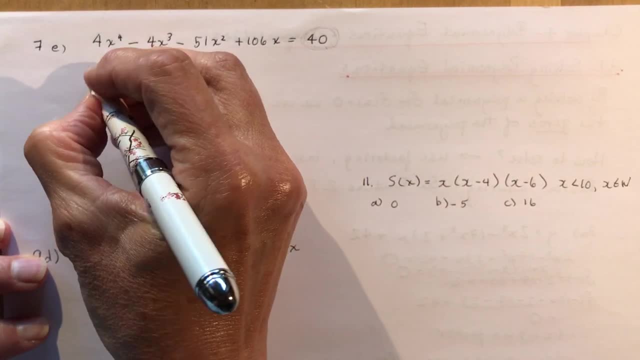 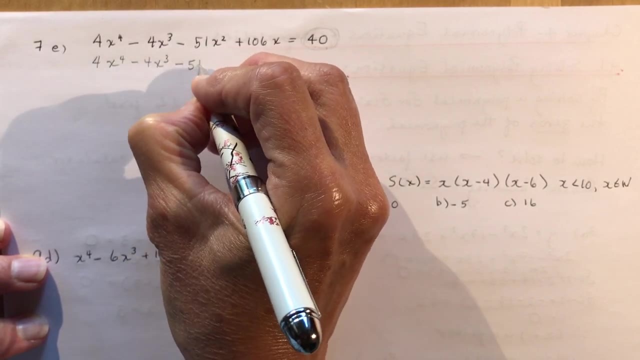 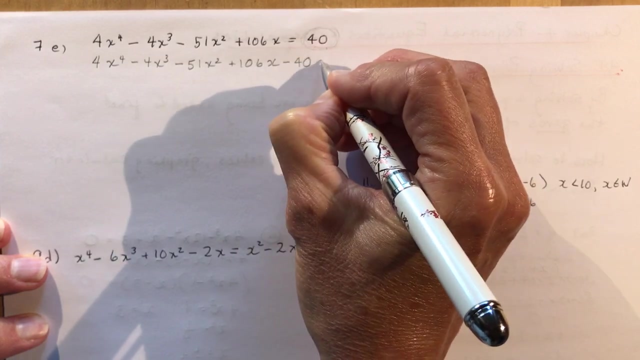 factoring. we need to bring this to the other side of the equation. so that should be your fourth. first step. um, it could be more than just one number over there. sometimes, in some word problems, you're asked to find when something is equal to something. you did that in your grade 11 course as well, so 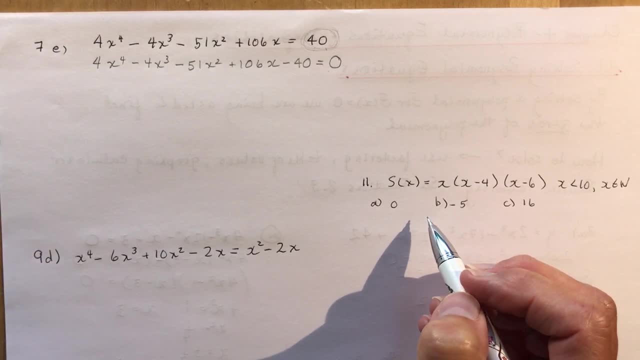 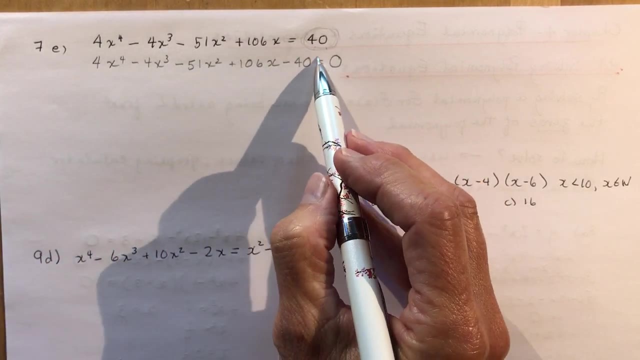 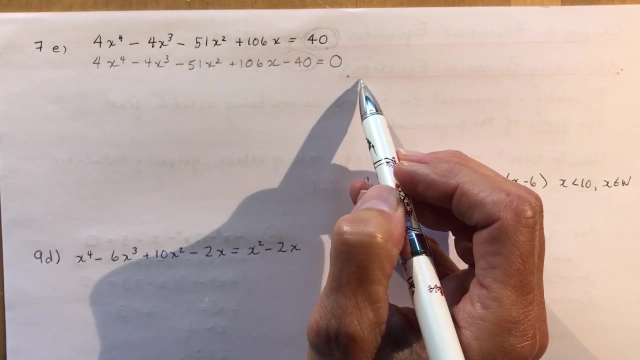 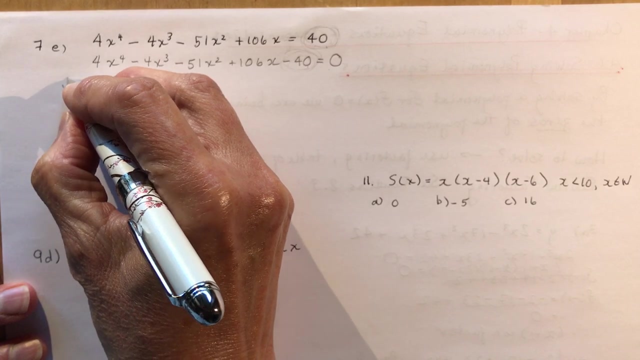 you set them equal to each other and now solve. so this one is kind of nasty. i mean, we've got all kinds of numbers here and we want to find something that is a factor of minus 40 that could make this equal to zero. so i have a little insider scoop here and we're going to check f at 2.. 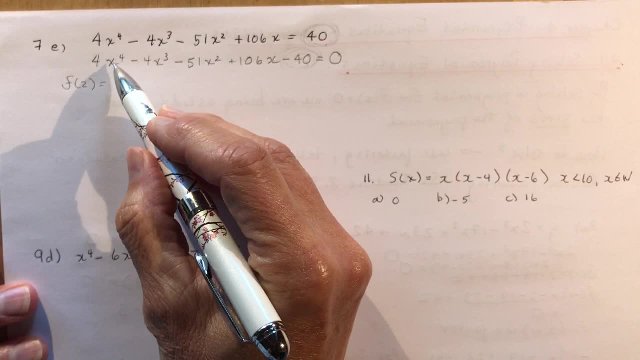 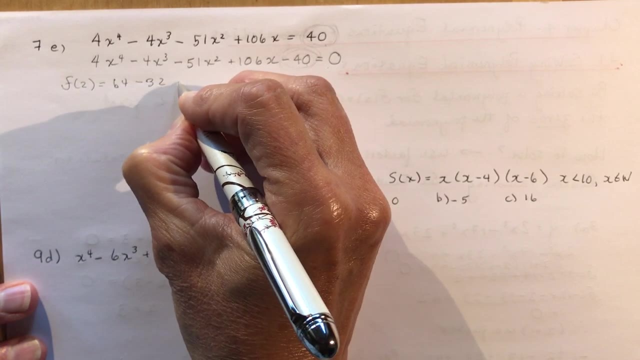 don't you wish you had insider scoop on your tests. so 2 to the power, 4 is 16 times 4 is 64.. We've got Freodorant for 4typ Jakobson to be square, so 2 times profile is 2 years. 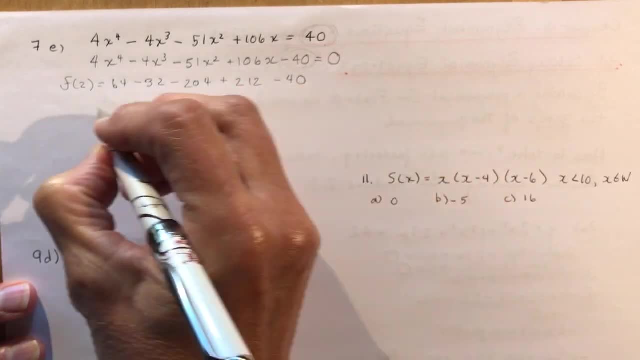 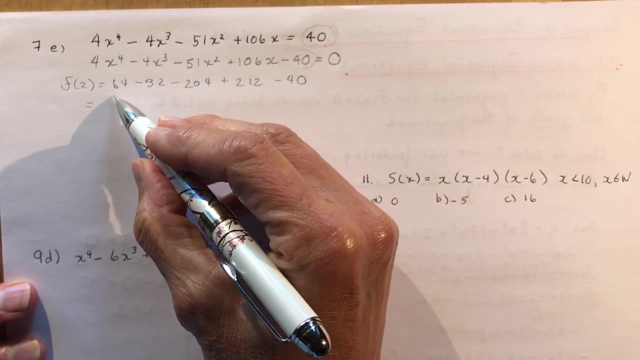 so i'm just going to break thosecessor problems down a little bit, because there should be something at 2 and 0 or 2.. here's the math. this is the formula 1, J, 4, 3, 0, 4, 4 and 2 plus 4, which is double 0 plus 4, 4, so 30 to. 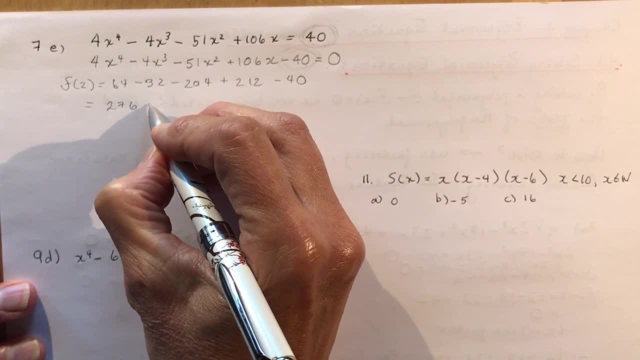 negative: 7, 0 and 3, so fl J 4, 4 minus 5 plus 14, 0 and 3, so that gets to 50, 2, 0, 0 minus 6 plus 9 plus 12 minus 30 and 3 minus 32.. 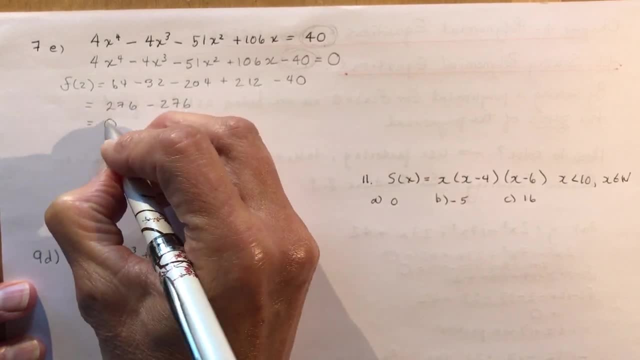 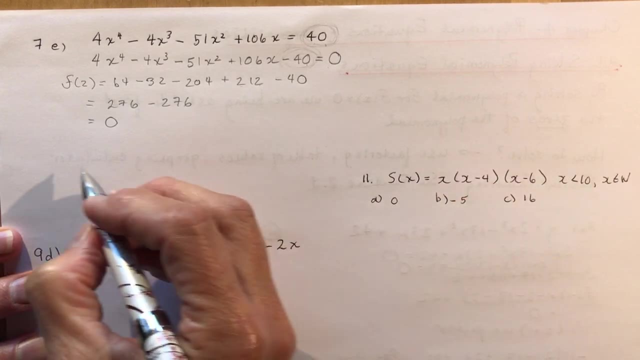 minus 276 in our minuses. So f at 2 is equal to 0.. So now what you have to do again is to use some synthetic division. This is the easiest way to do it, guys, So I write my 2 here. 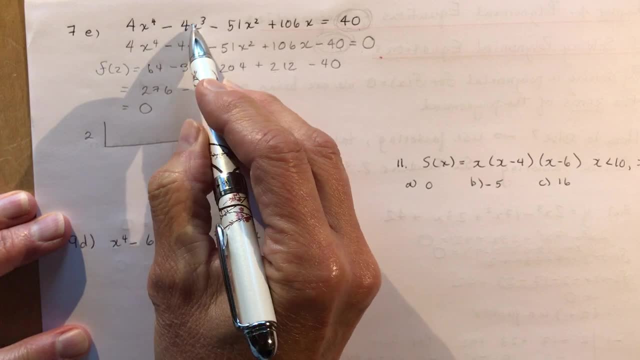 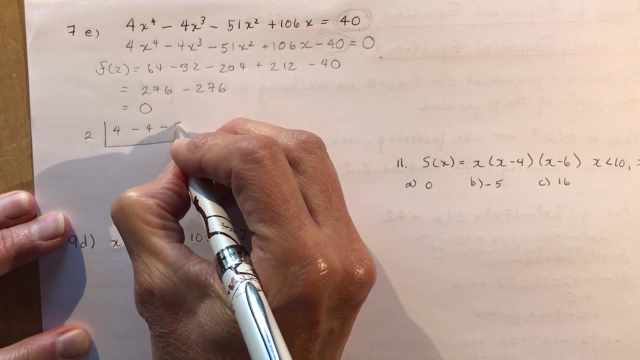 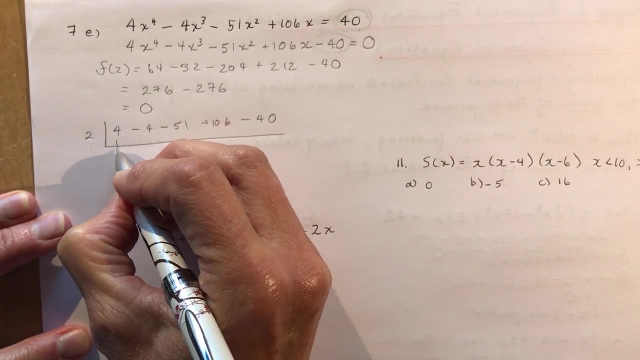 write this out and I write in all the numbers, the coefficients of all these and the 40.. Okay, so I'm going to put in 4 minus 4 minus 51 plus 106 minus 40. And if I'm right, then, like I said, 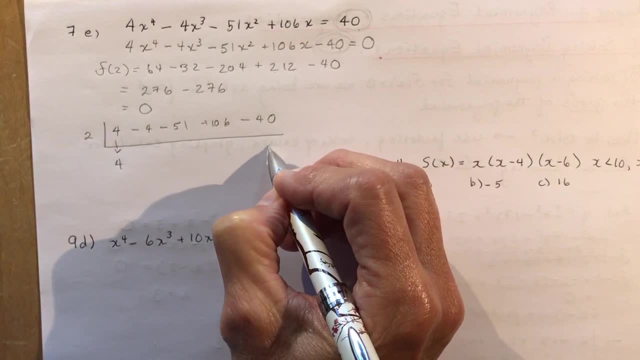 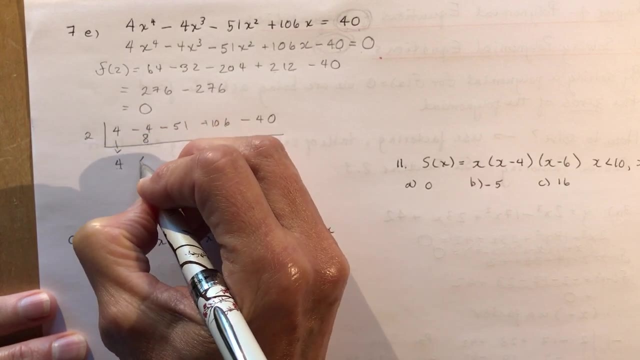 this is going to be equal to 0, the last term here. So I have 8.. I'm multiplying here again. Remember: 2 times 4 is 8.. I add them together Gives me another 4.. 4 times 2 is 8.. I add those. 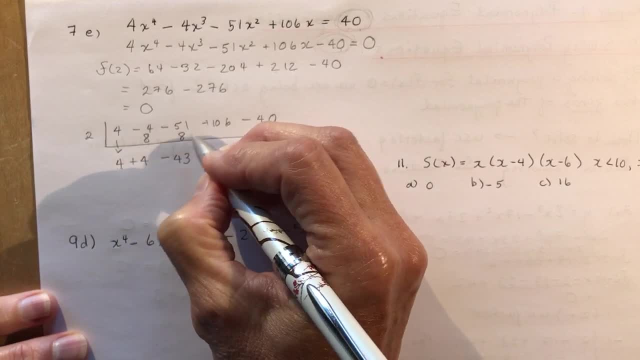 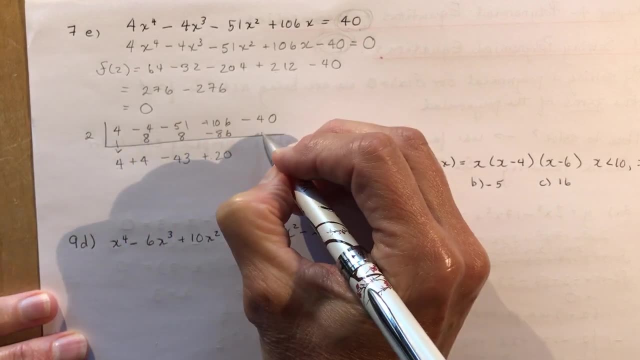 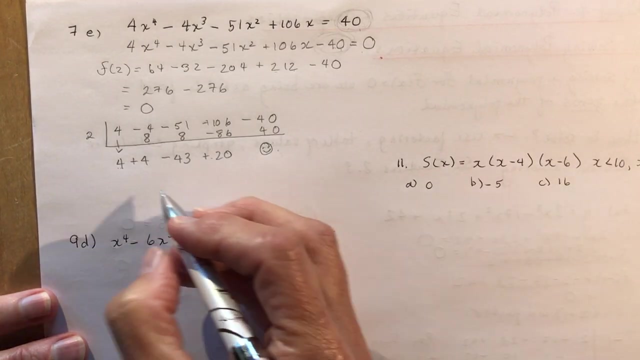 together, I get minus 43.. Times 2, again is minus 86.. I add them up, I get plus 20.. And 2 times 20 is 40. I add them up and I get 0. Again, if you don't get a 0, you've made a mistake. So this means now that I have 4x. 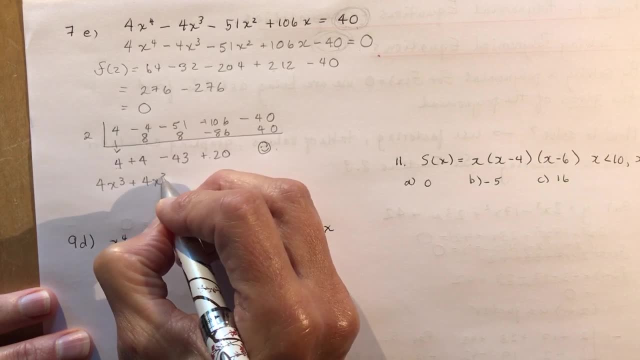 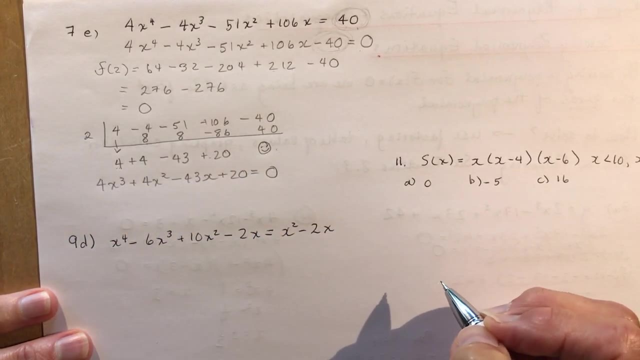 cubed plus 4x squared minus 43x plus 20, equals 0.. Okay so now I have 4x cubed plus 4x squared minus 43x plus 20, equals 0.. Okay so now I have 4x cubed plus 4x squared minus 43x plus 20, equals 0.. 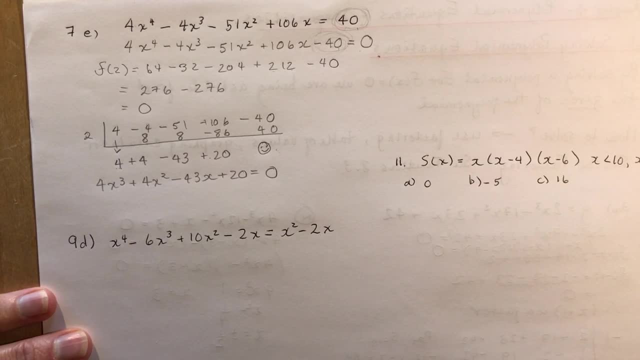 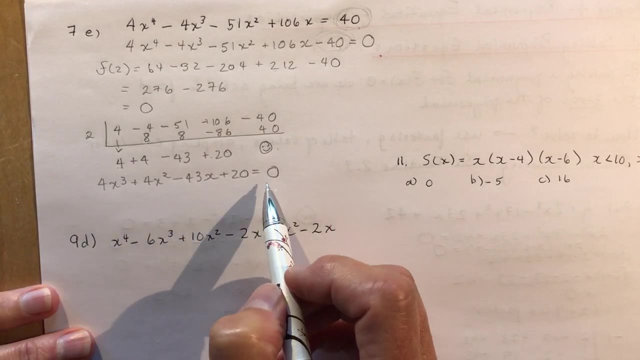 Okay. so I'm not quite sure what the question asked for your number 7.. Let me just check it here. in your textbook, Determine the roots algebraically by factoring. Okay, so now I have this and I have to go through the same process again, finding factors of 20 that might. 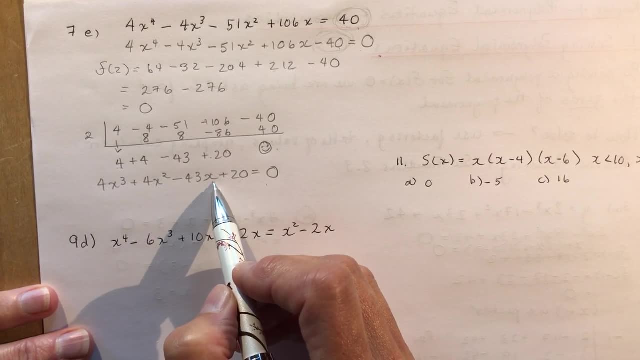 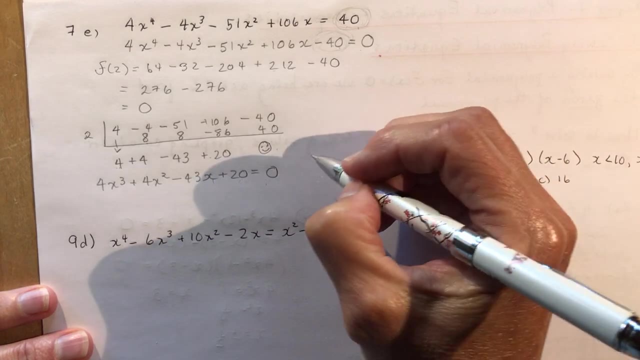 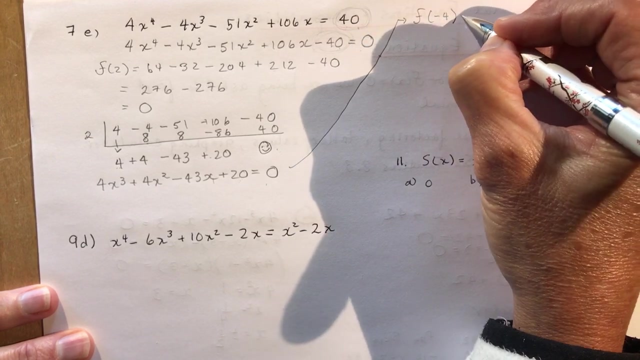 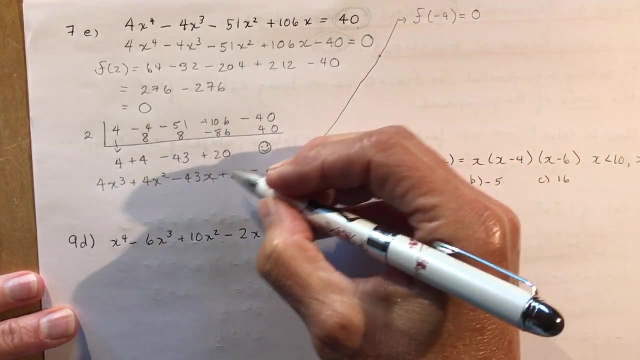 make this equal to 0. So I gain a little insider information so we don't spend a lot of time the whole time doing a bunch of practice rounds. F at minus 4 is going to work here. Do I need to write it all out? F at minus 4 is equal to 0.. You can do the checking on that I. 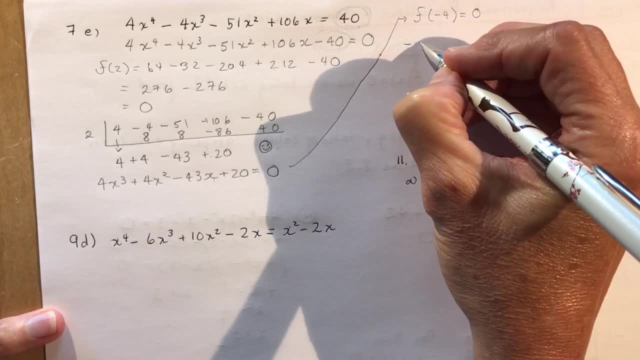 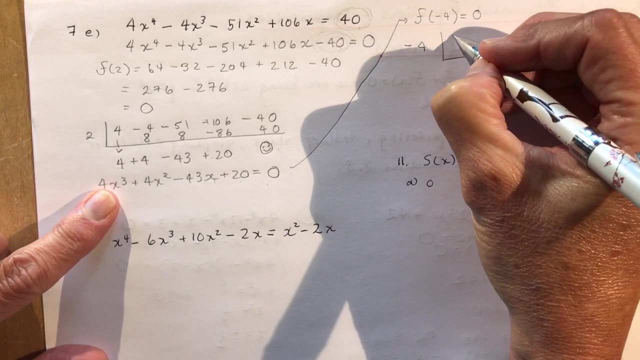 don't want to waste the time doing that. So again you have to do your long division. So you put in your minus 4.. You plug in the numbers from this one, So I have 4,, 4,, 43,. 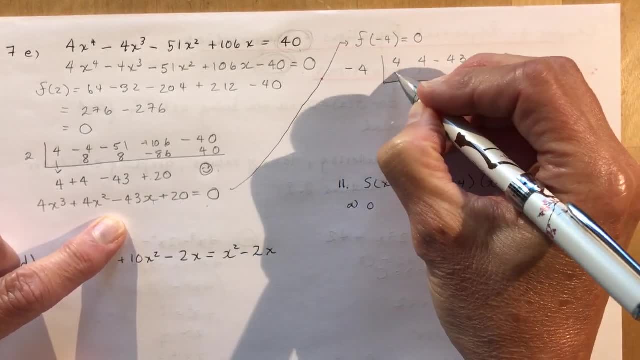 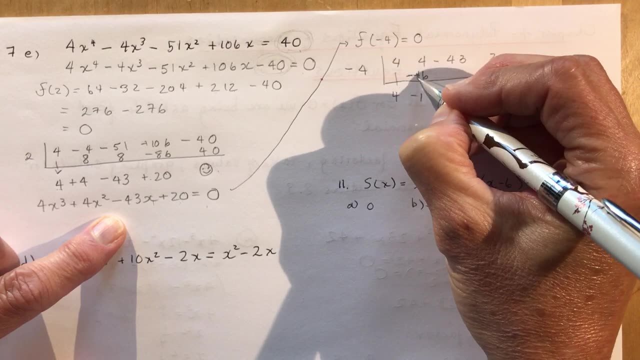 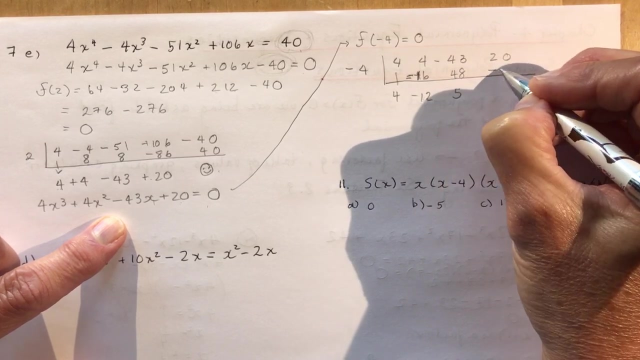 minus 43, and 20.. Bring down the 4. That's minus 16.. Add them up Minus 12. That's minus 16.. Minus 12. That gives me 48. Add it together, gives me 5.. Minus 20 gives me that fancy 0 again. 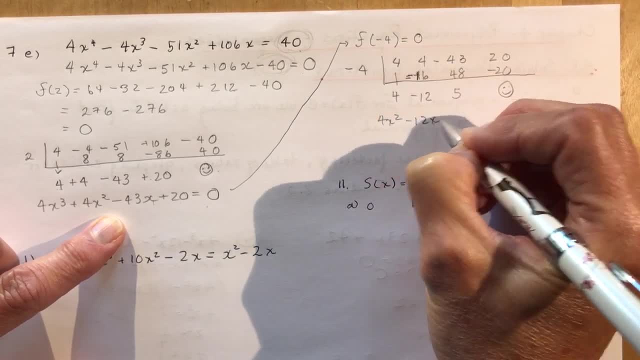 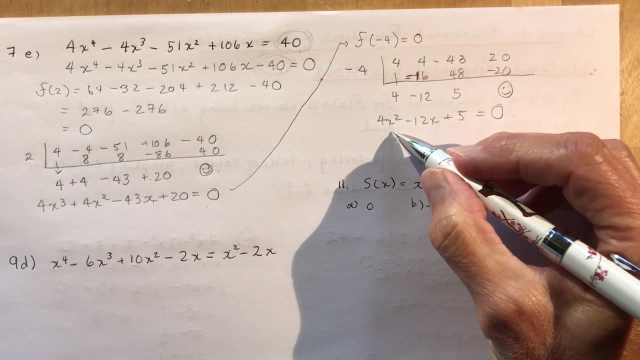 So now I have 4x squared minus 12x plus 5 is equal to 0.. And now it's a quadratic, So I can use my basic factoring skills. What multiplies to 20 and adds to negative 12?? Product minus 20,. 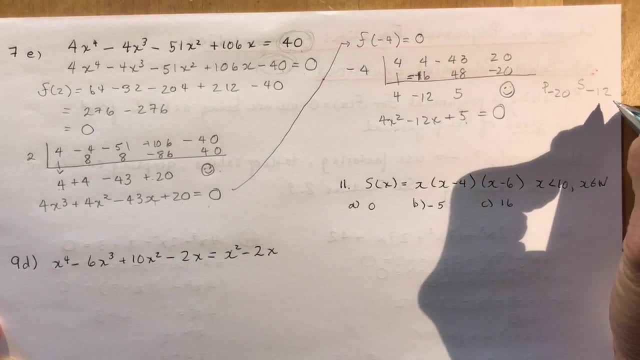 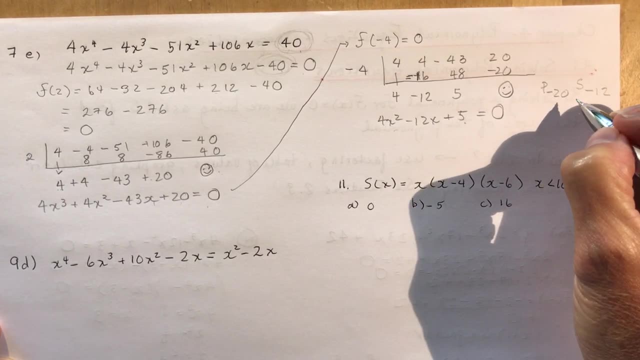 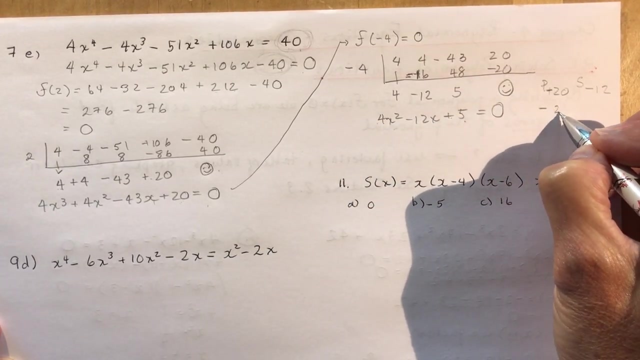 sum negative: 12.. 12 and product of minus 20.. 2 and 12, right, Or minus 2 minus 12.. It's a product of plus 20.. That's got me confused there. 4 and 5.. So minus 2 and minus. 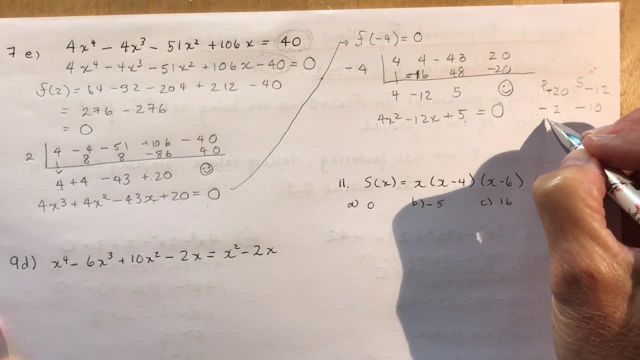 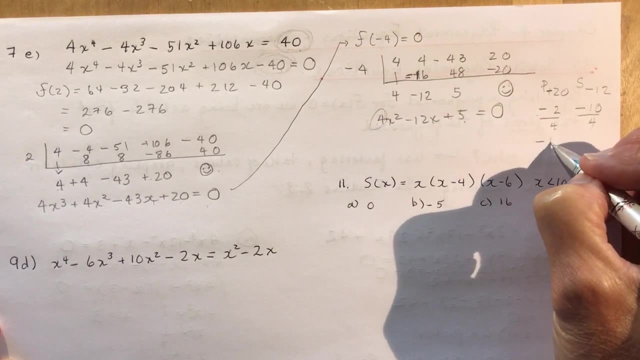 1.. Multiply to 20 and add to minus 12. And again I put them over the coefficient of x squared. So the first number here And I reduce, So that gives me minus 1 over 2,, minus 5 over 2.. So now that 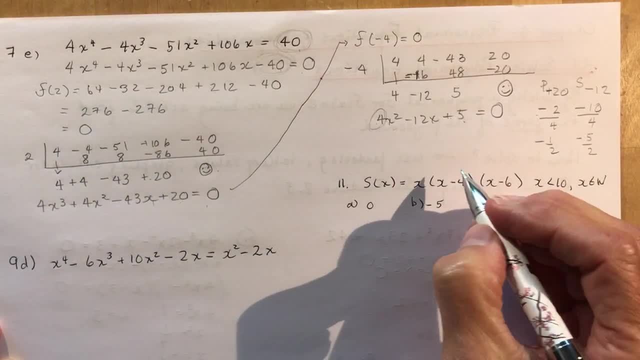 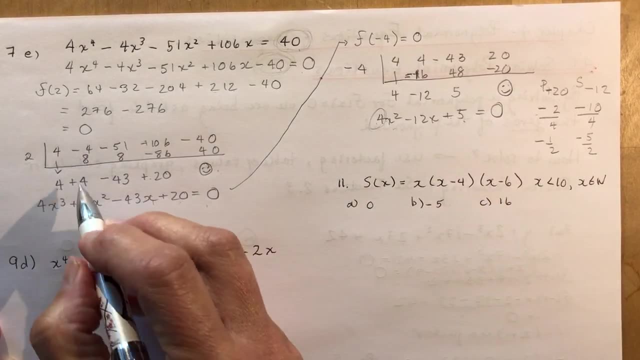 I've got this all factored. I can say what this equation is in factored form. I think this one just asks you to determine the roots. So you would say you had 1 here, which was 2, minus 4,. 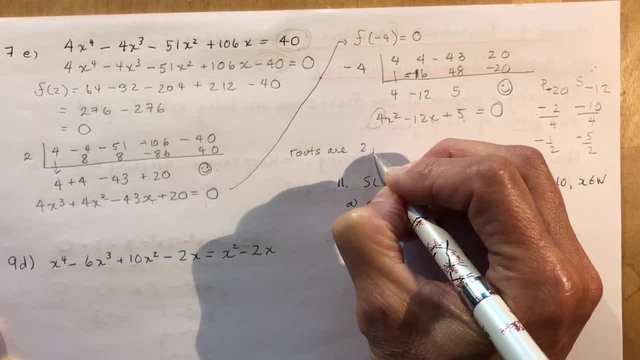 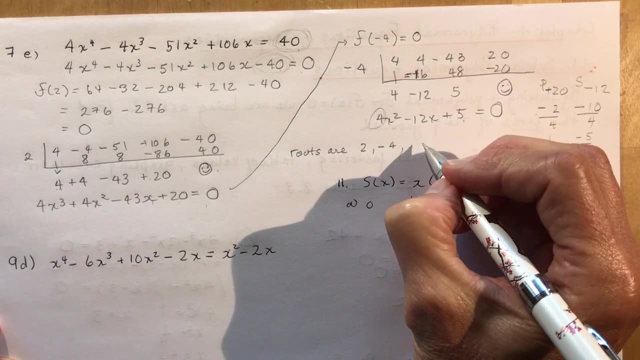 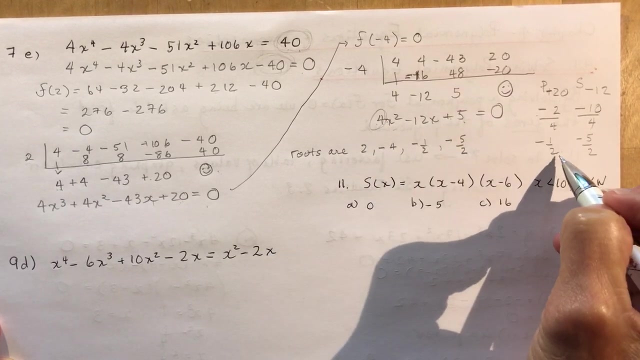 right. So I'm going to write: roots are 2, minus 4.. And this would be minus one-half and minus five-halves, Because remember, if you were to write this in here now, you'd say 2x minus 1.. 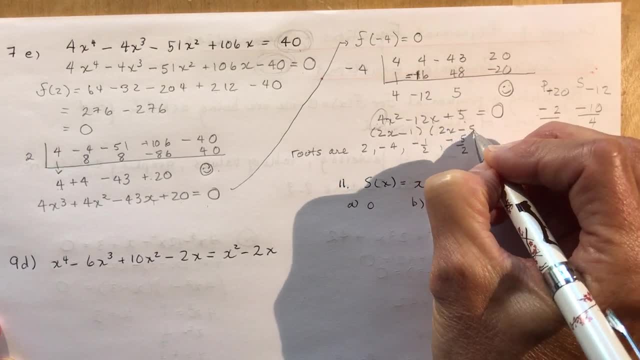 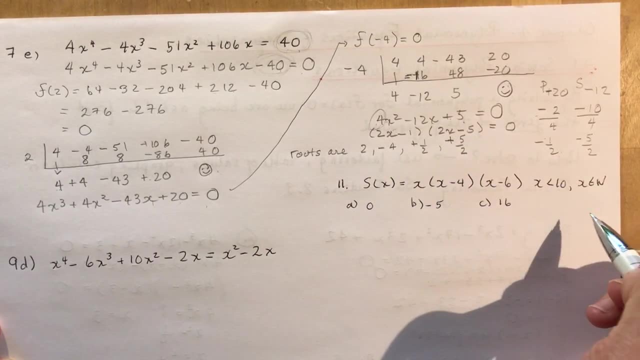 And this is: 2x minus 5 equals 0. Set this equal to zero. that gives you plus. So plus 1 half plus 5 halves the opposite sign of these ones, And that gives you all of the factors. So we've. 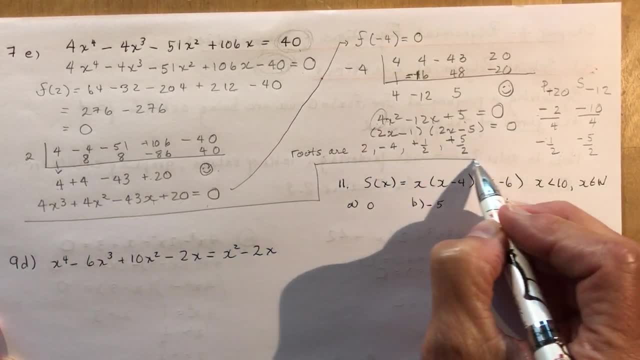 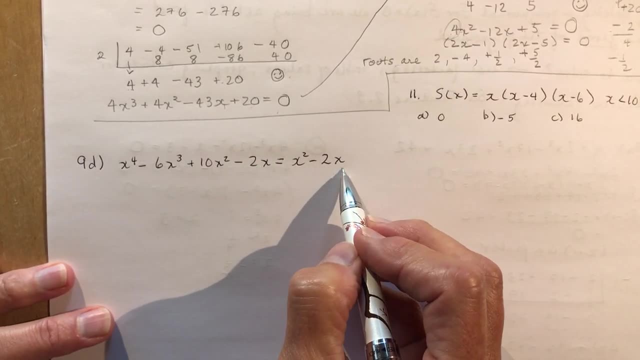 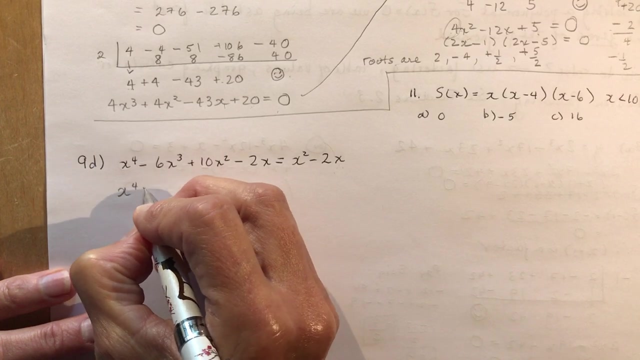 solved it wonderfully. Boom, boom, done. Okay, number 9d. So this is another example where things are on the other side of the equation, which means you need to bring them all to one side, set it to zero. So let's do this again: 6x cubed 10x. 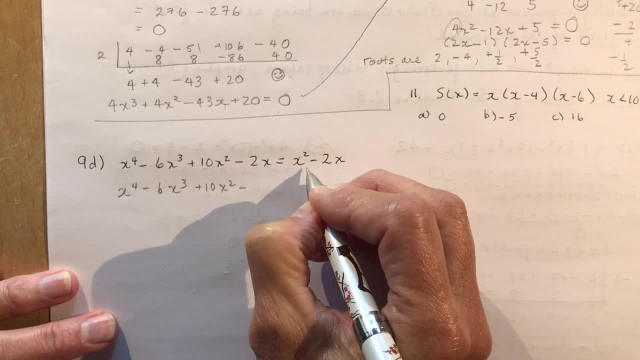 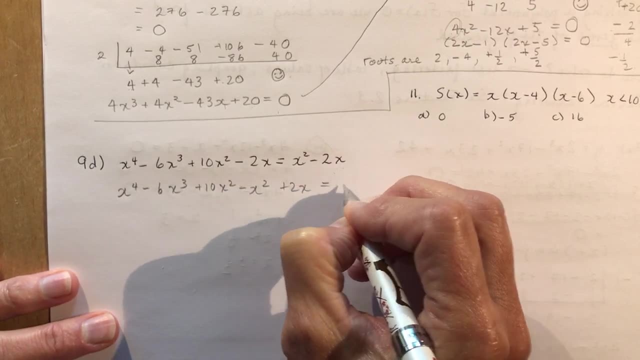 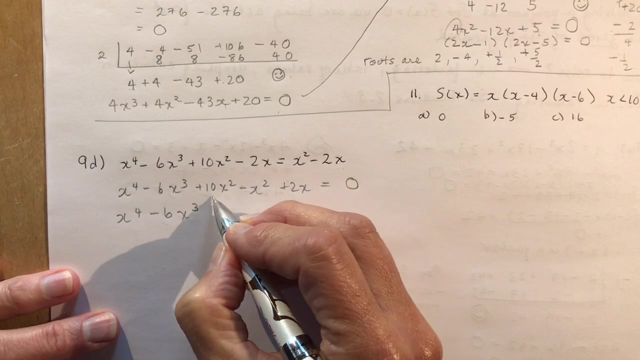 squared minus- I'm going to bring this over first- minus x squared plus 2x is equal to zero, So it gives me x to the fourth minus 6x cubed. Now, sometimes you can do this on a graphing calculator, if your teacher lets you. 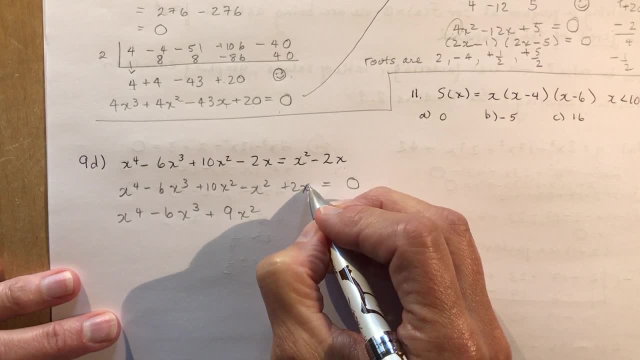 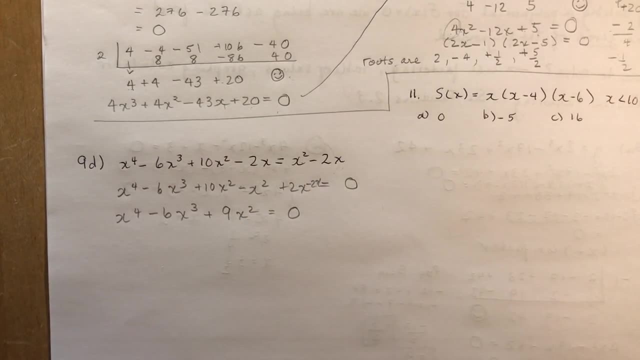 Okay, Okay, And I have a minus 2x here too, So those canceled out, Okay. so now what am I going to do? I've got these x to the fourth minus 6x cubed plus 9x squared equals. 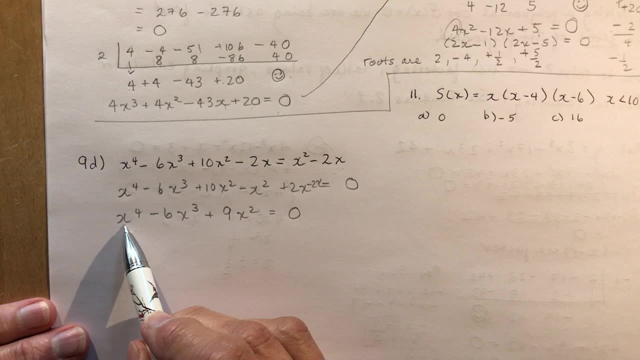 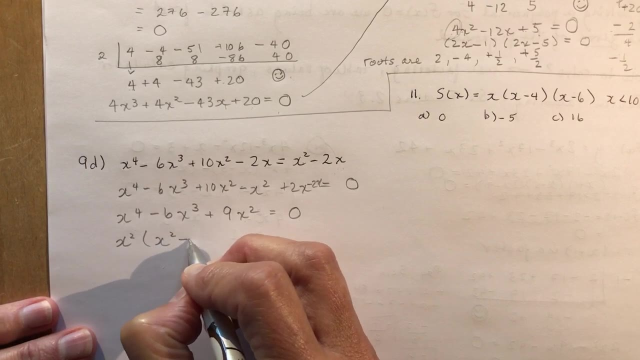 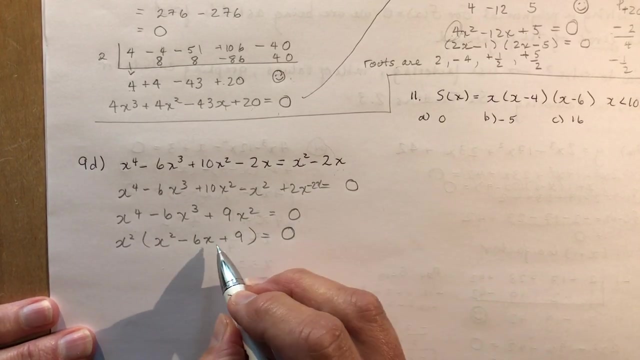 zero. So I don't have a constant, but I do have a nice common factor here. So that would be x squared right. And look, it's going to leave me with a nice, simple, easy to factor trinomial. Perfect square actually. So this is going to be x minus 3.. So x. 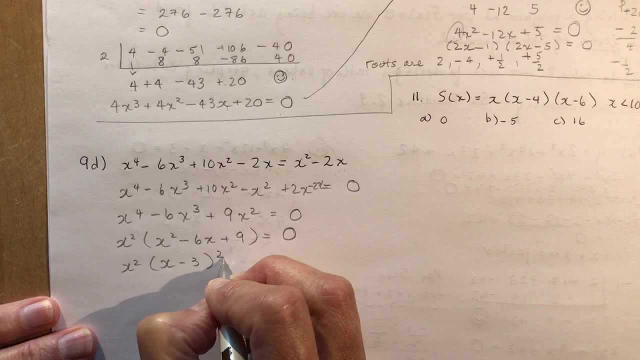 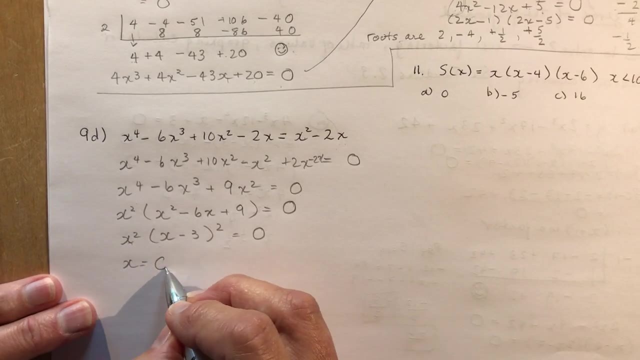 squared times, x minus 3, squared is equal to zero And x is equal to. don't forget, this one would be zero. right, This is zero And this one is three. Okay, so the last question I'm going to do with. 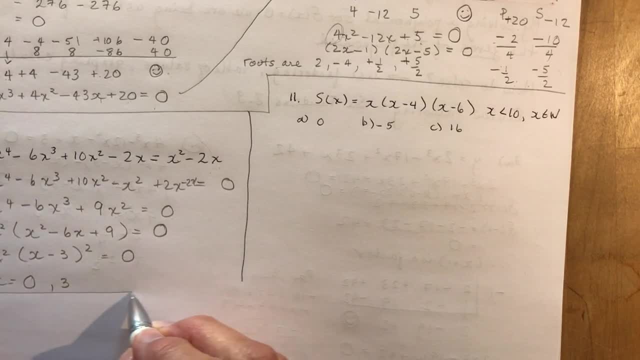 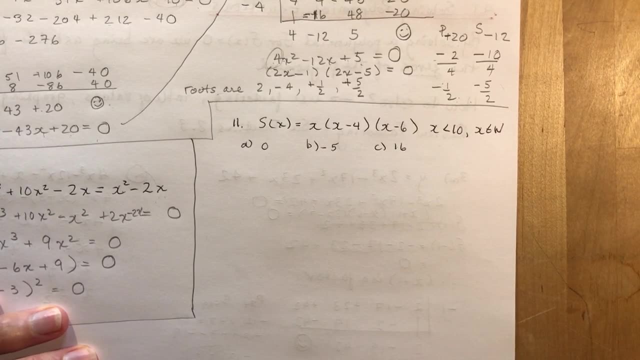 you is my favorite one because it's going to be x squared times x minus 3 squared. So I'm going to do this. This is a really funny name. I don't know who makes up the names for questions in the textbook, but they must have had fun making this one up, And it's a company, a family, called the. 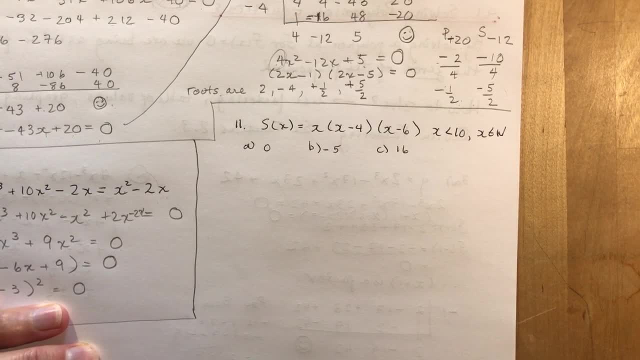 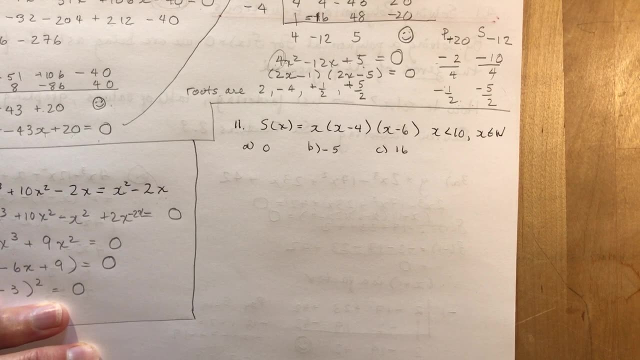 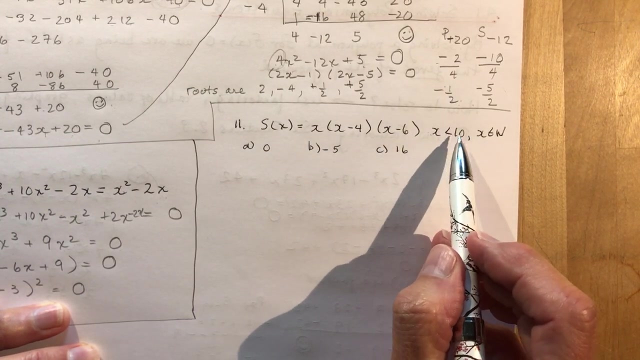 Sickle Lickty family members are very competitive card players. They keep score using a complicated system that incorporates positives and negatives. Maya's score for the last game night could be modeled by this function, which is this one here. So it says x is less than 10,. 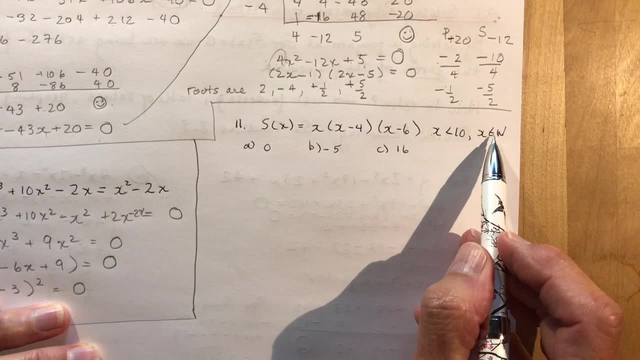 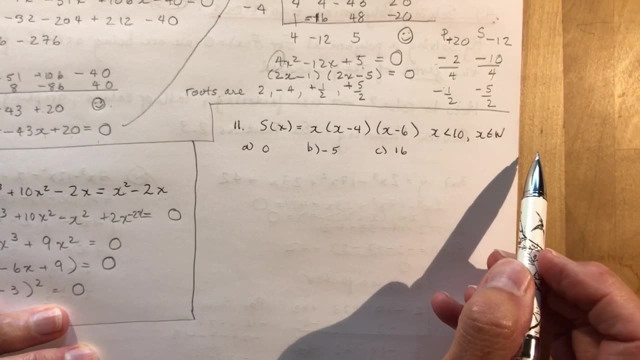 which means they only played nine games. And x is an element of w, that's whole numbers. So that means 1,, 2,, 3,, 4,, 5, 6, you couldn't play half a game, they played all full games. So question A: 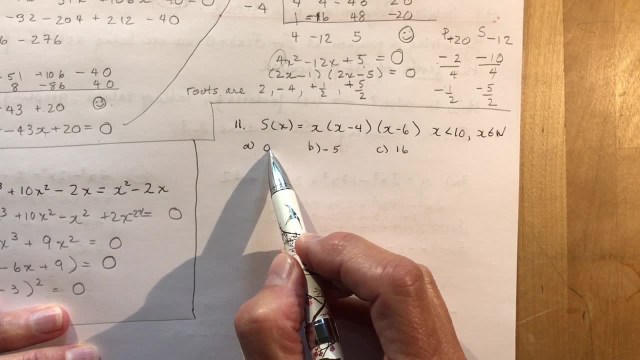 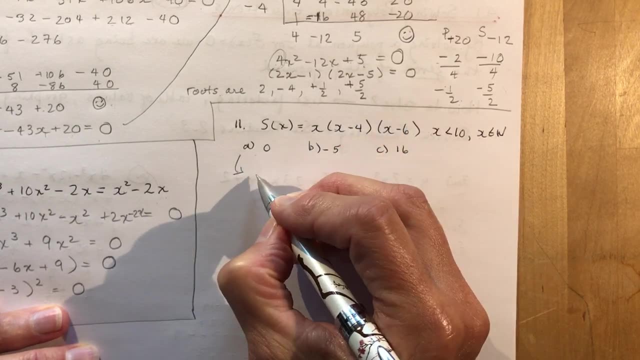 says: after which game was Maya's score equal to zero? Well, that's your easiest question to answer, because you're just wanting to know what are the zeros of this function. So they are 0,, 4, and 6.. This one is irrelevant. 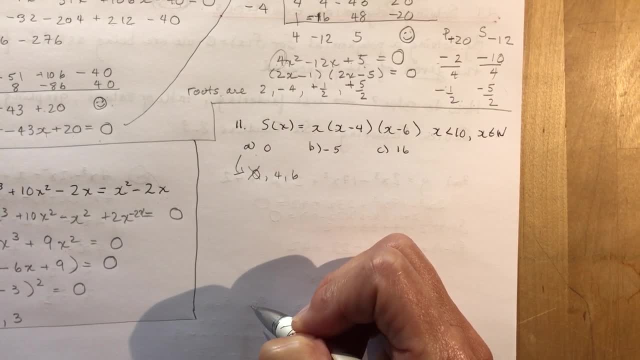 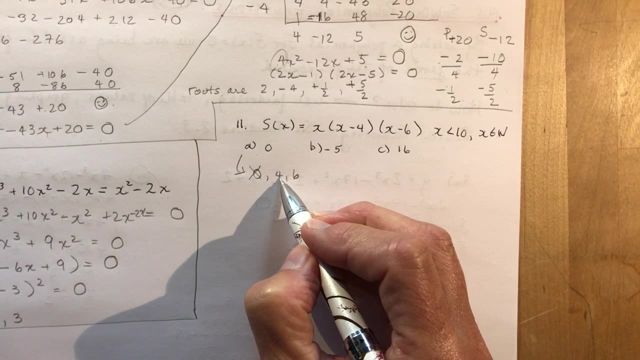 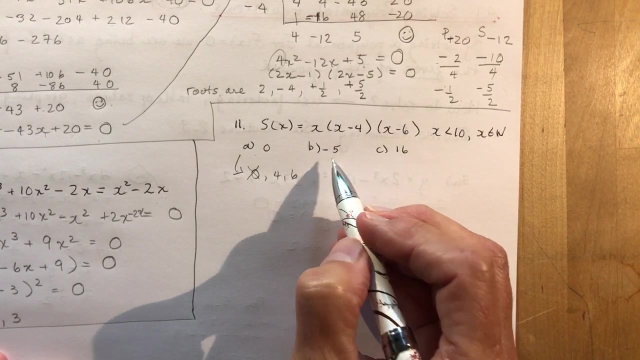 This one is irrelevant to the solution because you don't say: well, before they started she had a score of zero. Well, everyone did So. she had a score of zero. after the fourth game and the sixth game. Question B says: after which game was her score minus 5?? So this time you need to set the 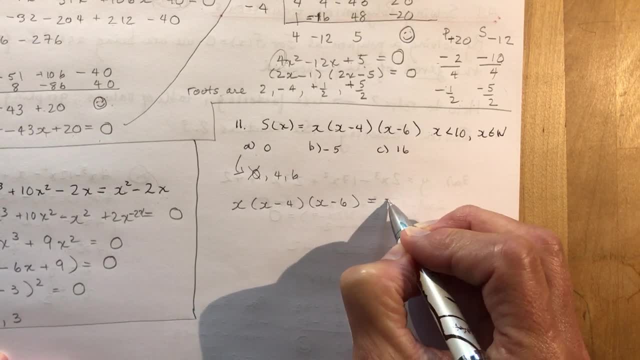 score to minus 5.. This is the score at game at some point. So this is the score at game at some point. So this is the score at game at some point. So this is the score at game at some point. 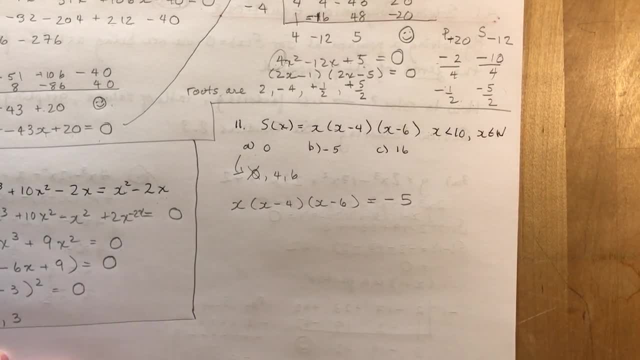 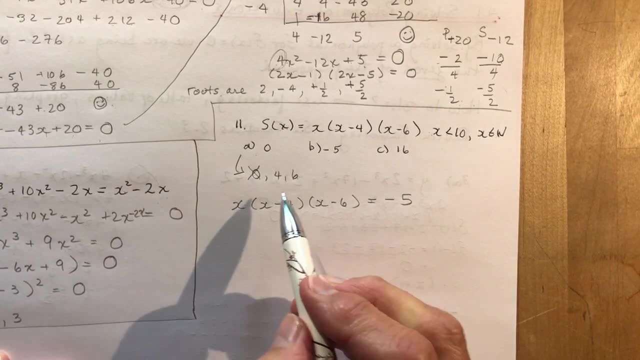 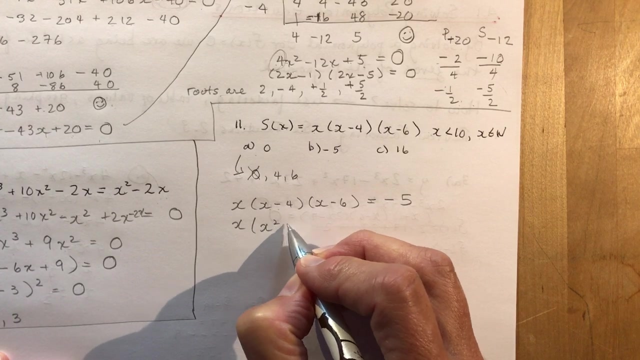 It's some game number. So in order for you to solve this, you're going to have to expand it and simplify. So I need to expand this question. So this is x squared minus 6x minus 4x, So x squared minus 10x. 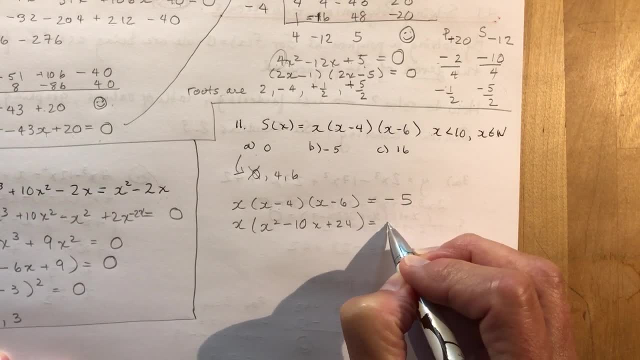 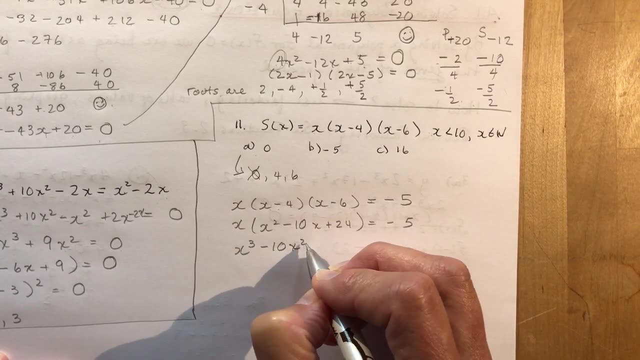 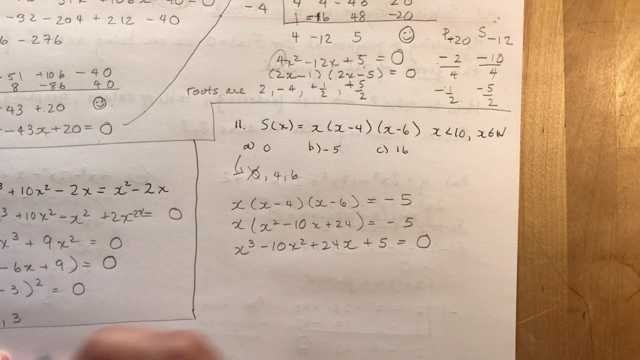 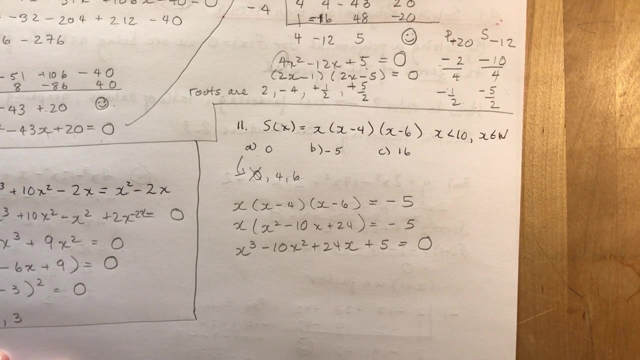 plus 24 equals negative 5.. So I've just expanded this and I'm going to multiply by an x and I'm going to bring the five over to the other side: equals zero. Okay, so when was her score minus five? Well, you might want to guess that it was probably sometime between game four and six. 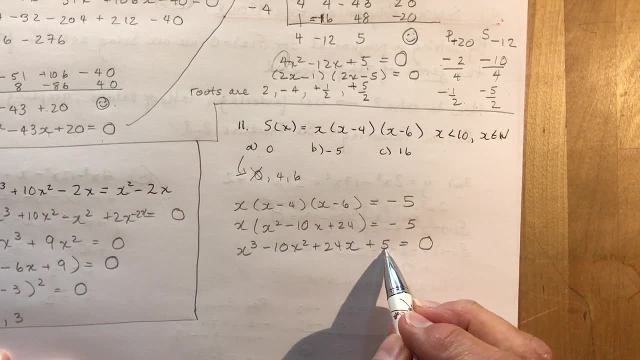 and the only well. you could try one, because the only factors of five are one and five. You put in one, you're going to get 1 minus 10, that's minus 9, plus 29, that's 20. so that's not zero. So F at 5. 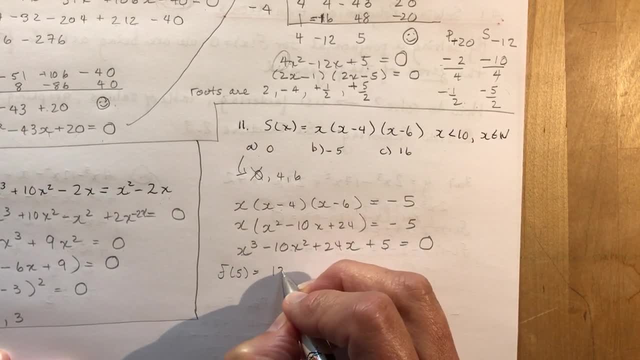 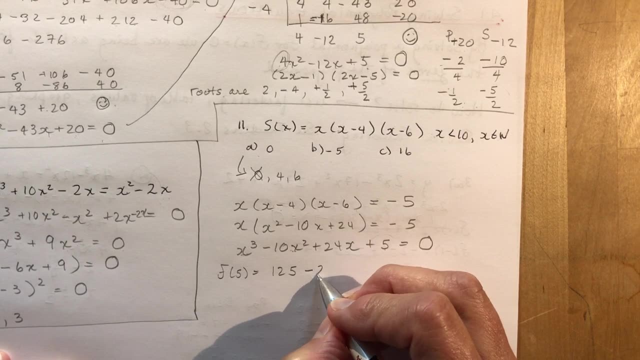 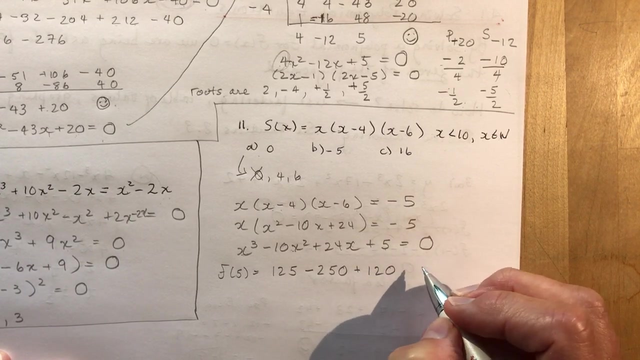 let's try F at 5.. So 5 cubed is 125, 5 squared is 25 times minus. 10 is minus 250, 5 times 24 is 120 and plus 5.. So you can see I have. 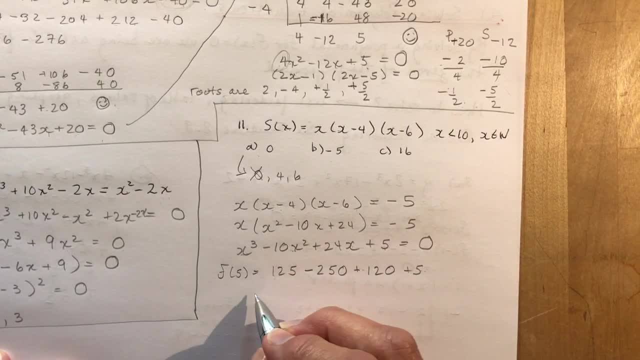 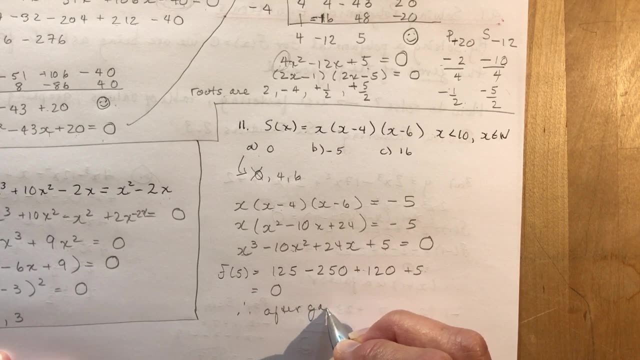 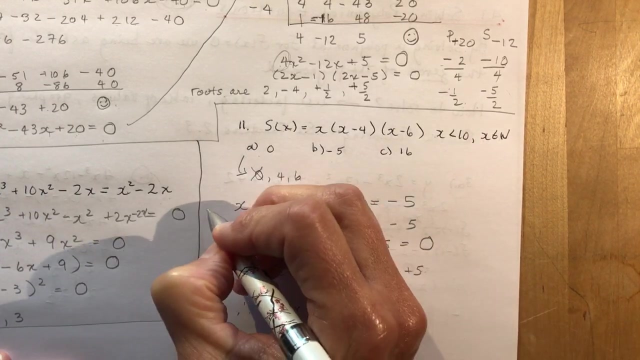 20 and plus 5.. So you can see I have. So you can see I have 125. 125, that's 250 minus 250 is zero. so that means after game five or at game. after the fifth game. her score was minus five. that's your b part and see. 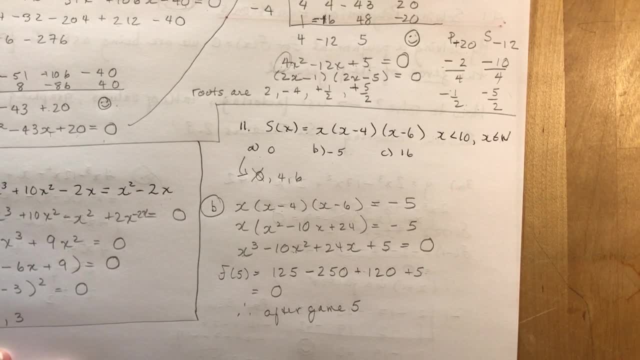 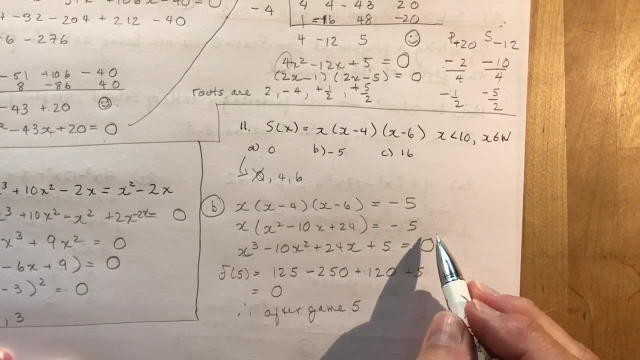 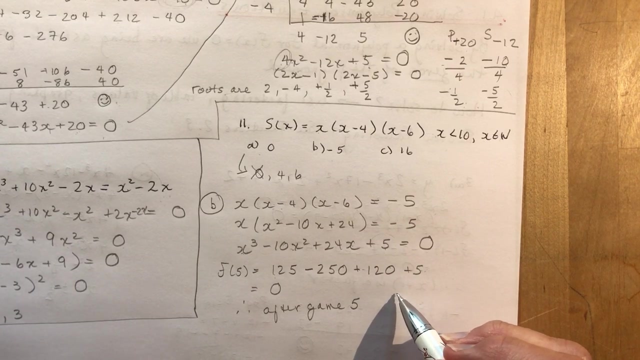 when was it equal to 16? well then, you're going to have to do one more calculation here, so you're going to set this equal to 16. i'm going to let you finish that. it's not difficult now. so you should be able to set it to 16 and again solve for, solve for x. now the last part of this. 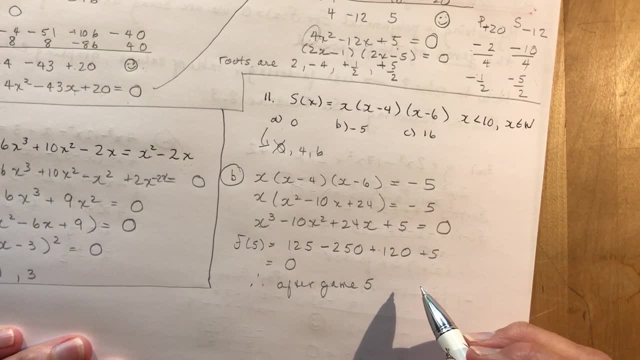 says, draw a sketch of the graph of f, of s at x, if x is an element of real numbers. and why is this not a good model to represent my score during the game night? and the reason for that is because you're going to have to do a little bit of math and you're going to have to do a little bit of. 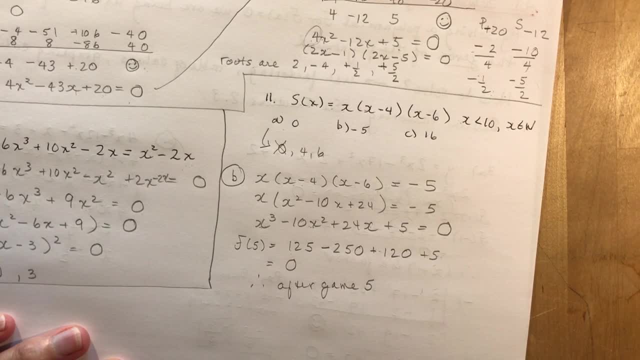 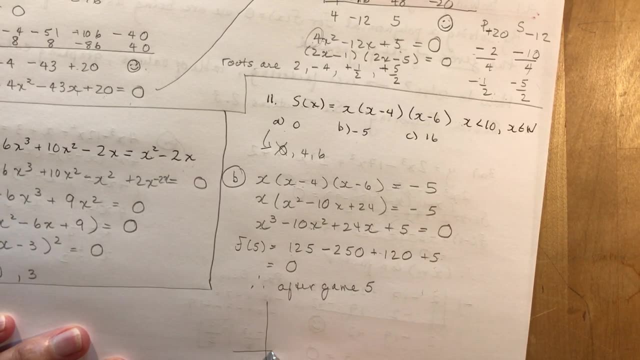 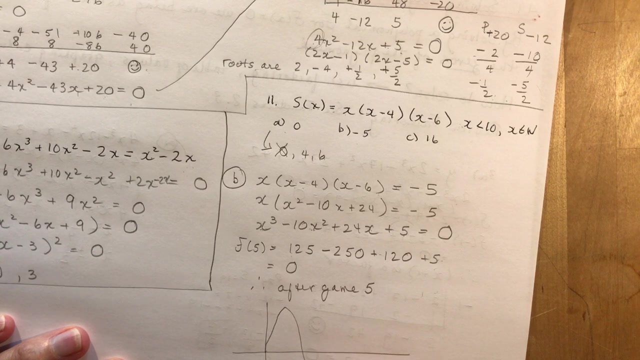 math and you're going to have to do a little bit of math and you're going to have to do a little bit of it shows game values when you do real numbers. so i'll give you a quick sketch of what it should look like. so it started real numbers, it started at zero and she, her score, kind of goes like this: